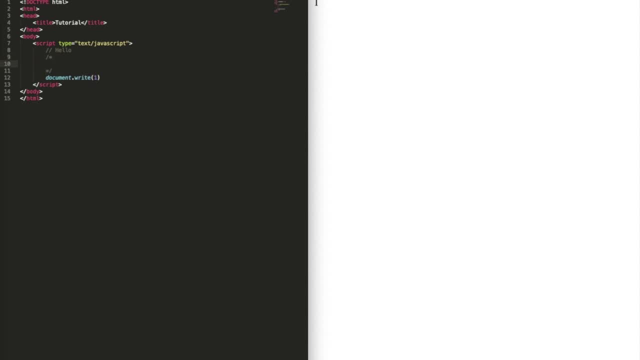 a multi-line comment. okay, So you can write multi-line comments. Okay, So yeah. and then there are different data types, for example int, float, string and Boolean. okay, So an integer can either be 5, or 8, or 9, or 101,- sorry, 1001, or minus 200, 2003,. 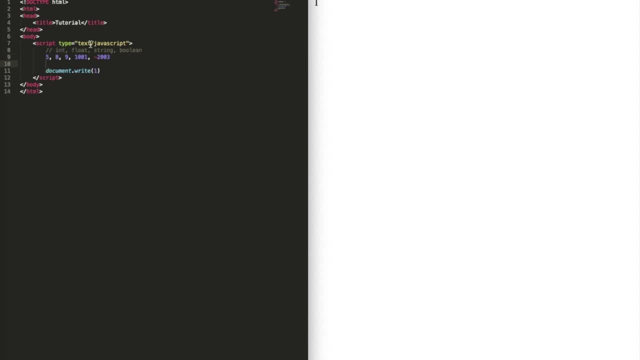 okay, It's basically anything without a decimal okay. So even 5.0, right, It's basically anything without a decimal, okay. So if you put 5.0,, that would be a decimal, okay, And a quote is a decimal. so 5.0, that's a decimal, and 5.03 is also a decimal and minus. 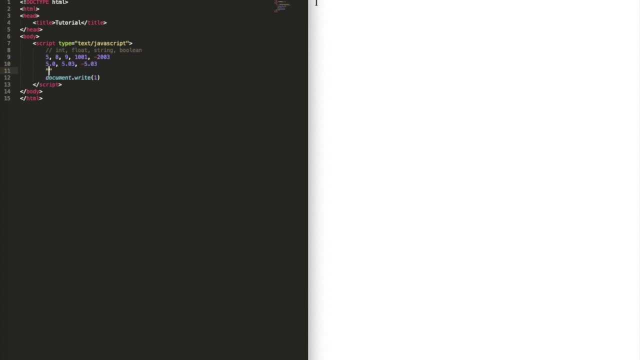 5.03 is also a decimal, okay. And then string is anything, with two pairs of quotations at the and then also at the start. so, as you can see, first you put a quotation and then another quotation and you can write anything here. 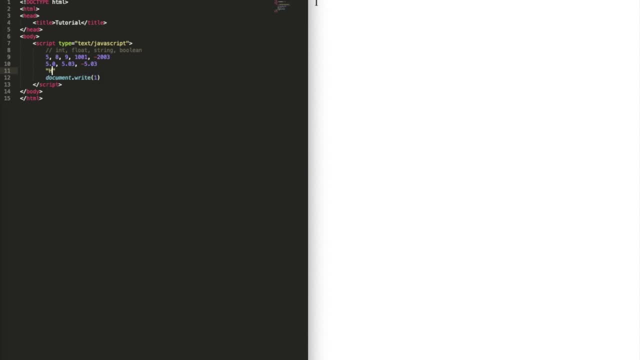 For example, hello world And a string can also only have numbers, so like 880.5, blah, blah, blah, okay. And at the same time it can also have a letter, so B Boolean, yeah, okay, whatever. 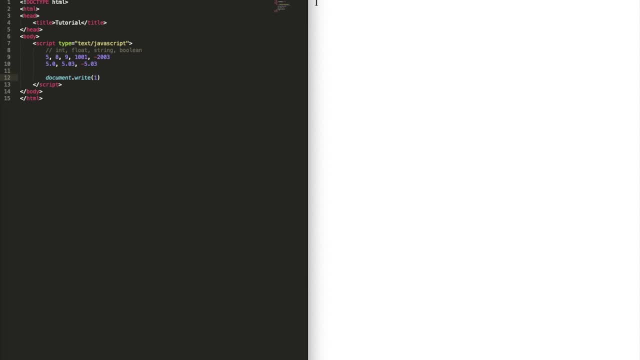 So it can. it's basically anything with two quotations, okay. And now Boolean is. it only has two values, which is true or false. okay, So those are the main data types, and then you can also print these data types. so for 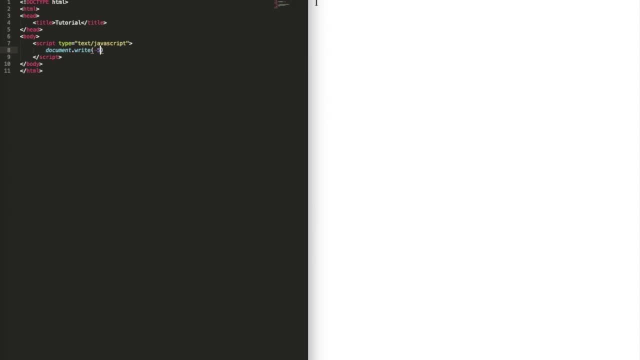 example one we just did: that's an integer, minus five is also an integer, and then a float minus 100.3,. okay, And then you can also print out a string so you can do hello world, and then you can. 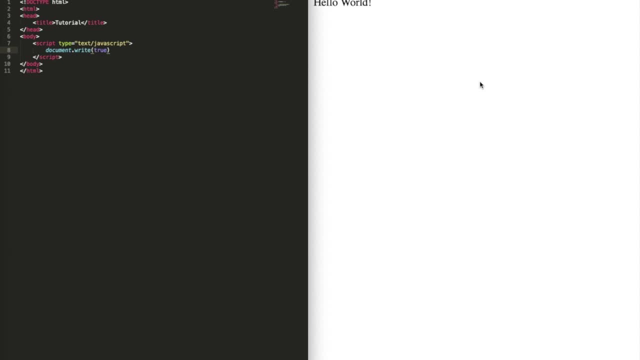 also print out a Boolean. it's true, okay, But if you print out a string, for example, and do and do not include the quotations, then it's going to give an error and you can inspect the element or show the page source. 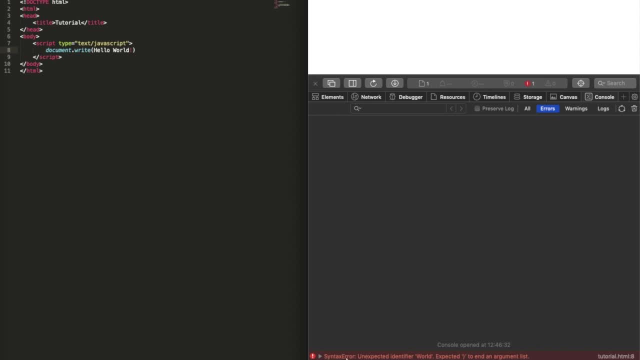 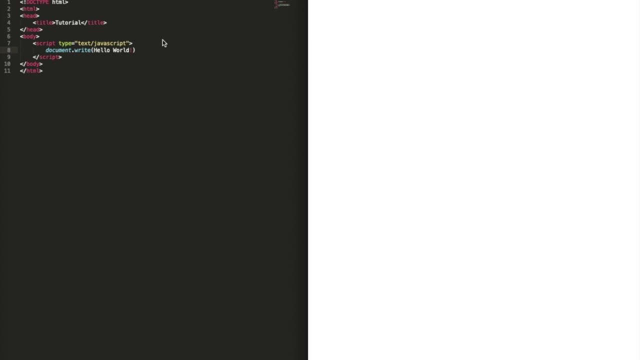 and you can go here and then say: syntax error, unexpected identifier, world expected quotations, okay. So this is why you need quotations. okay, So now you can do hello world, alright. So that's the basics. and also, whenever you end a statement in JavaScript, you always 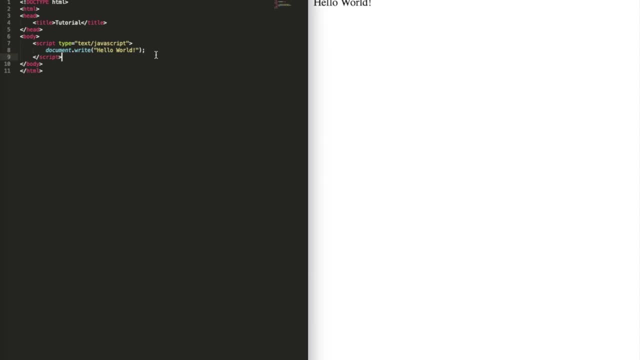 need a semicolon, Okay, And now what you'll need to do is we're going to learn arrays, okay. So first we're going to learn variables, so a variable can have any of the data types, so it always starts with var, okay. 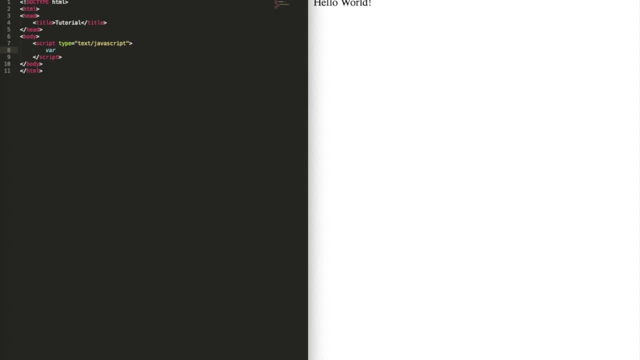 So var, and then the name of the variable, for example x equals two, or it can either be five, and then you have to end the statement. so this is an integer, And then it can also be a string, for example hello, and then it can also be a flow for. 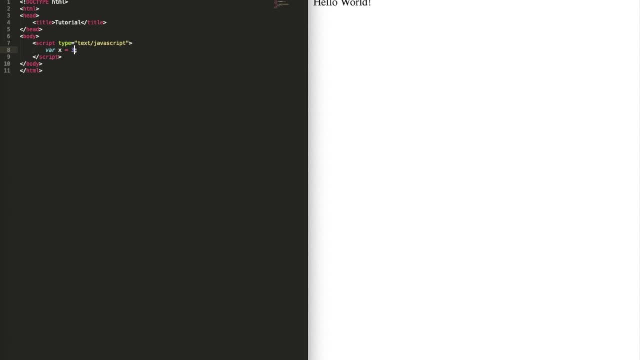 example 3.1415,, and then it can also be a bool: okay, True. And then you can also print a variable. so documentwrite x, sorry x, and since yeah. so you just put x there and then it will print out true. and then if x is five, then 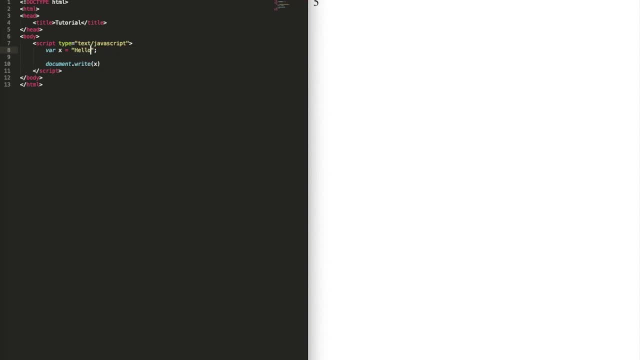 it will print out five, And if x is a string, so hello, Okay, So, and then you can also change the variable. so var, sorry, and then x. so, like whenever you change the variable, you just use the name of it. so you're going to use var, okay. 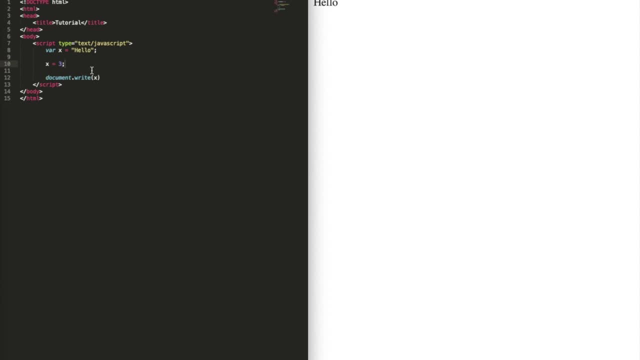 So x equals two, twos, okay. So now x is going to be equal to three, or it's going to print out three, okay. So just to see the change you can also do, documentwrite x up here And then first it will print out hello, and then it will print out three. 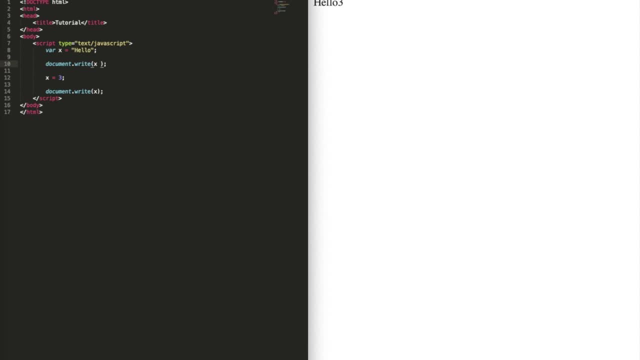 And with HTML you can actually, you can actually also give a break. so x plus and then in quotations, vr with a tag. that means break in HTML. okay, So first it prints out hello, and then it changes the variable and then it prints out. 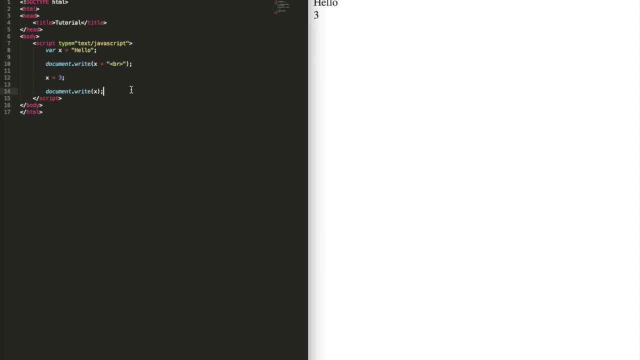 three, because we changed the variable into three. okay, And now you can also increment the variable which is adding our variable. We're subtracting it, so you can do x equals to x plus three, so like it basically changes the value of x plus three, okay. 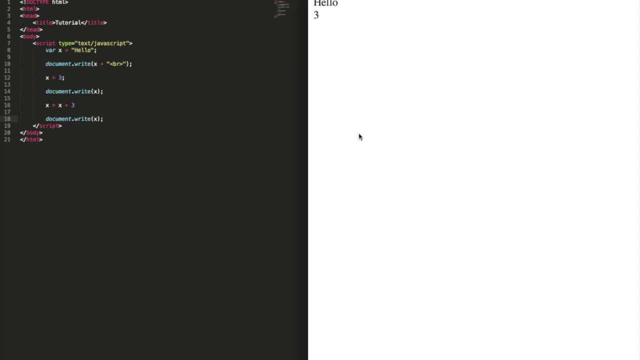 And then documentwrite x and I'll give six, okay, Oh yeah. and I always have the plus, be all, okay, Yeah. And then you can also subtract it, so you can do: x equals x minus three, so it goes. 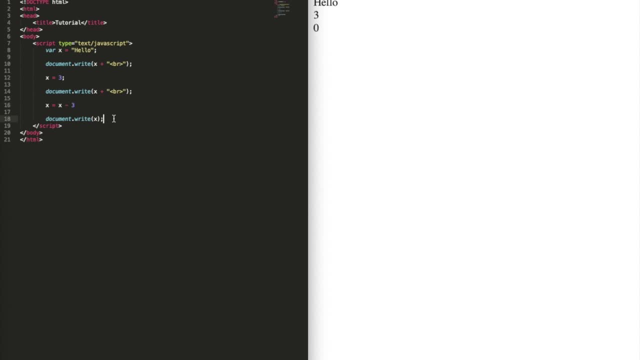 zero, okay. So first hello, then three, then zero, Okay. And you can also multiple variables, so you can have var y equals zero and you can print out y. okay, You can also change this to a true and it will print out true, okay. 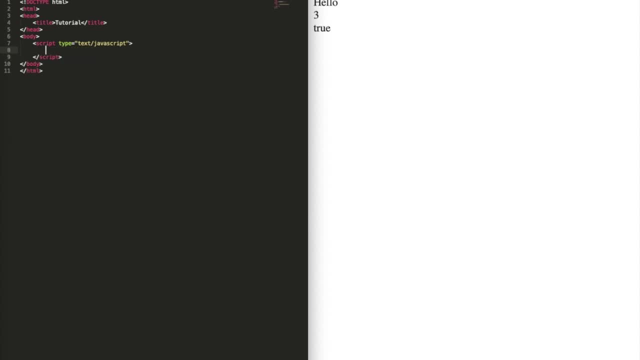 Now we are going to be covering the other data types. The first one is going to be called an array. okay, An array is going to. since it's also variable, we're going to start with var, and then the first one is going to be called an array. 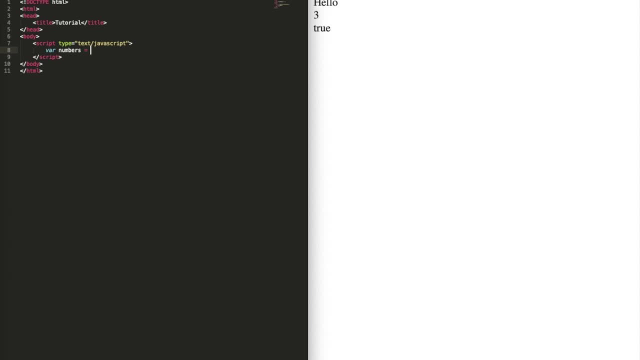 So let's say, let's say numbers okay, Equals okay. Now an array is kind of like a list okay, So like it has a list of items okay. So, for example, you can start with one and then you have to. this is the first element. 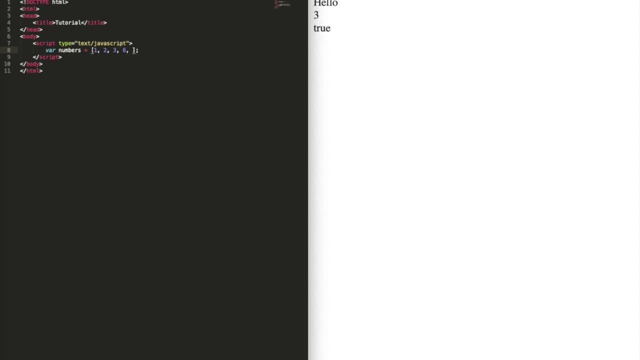 one and then two and then three and then five, so six and then four and then nine and then zero and then eleven. okay, So these are different numbers in the array and each of them have their own index. 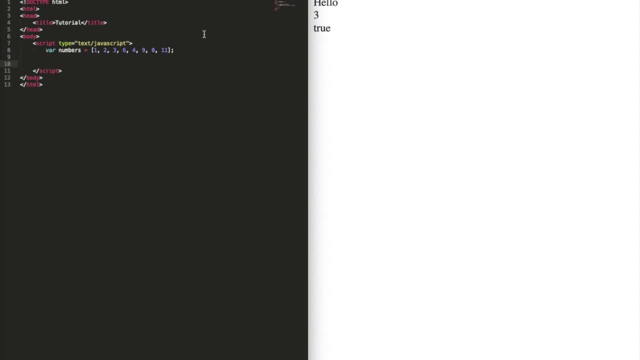 okay, and I'll tell you what that means. so, um, yeah, so an, uh, an array can have, like uh, not only numbers. it can also have a string, so let's say nine. you can also have a boolean, so let's say true. it can also have, uh, the floats of 5.03, and it can also have another array inside. so, um, 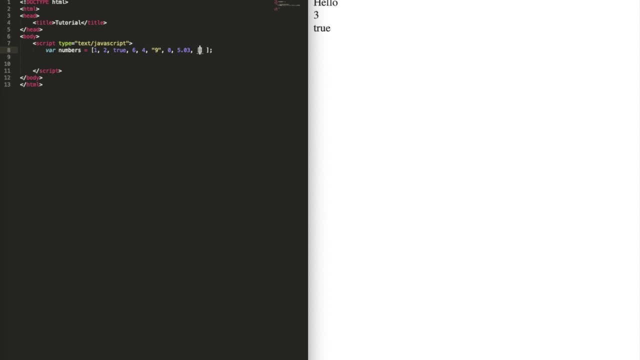 see, whenever you create an array, you always use these two square brackets and then inside you can put other things. okay, so like the first element is one, then two, then true, then six and four, then um, a string that is nine and then zero, and then 5.03, and then another array which has three and 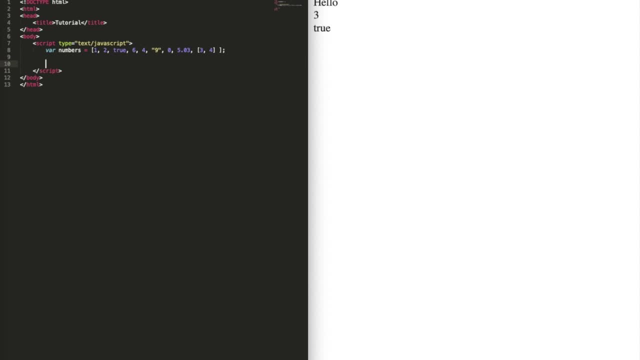 then four. okay. so, uh, I'll just tell you how to activate each element. so whenever you document it, right, if you print out the whole array, then it will print out the whole array with um, uh, with the columns. but if you want a single element, then you can do, uh, you can access it by using square brackets, like that, and then um. 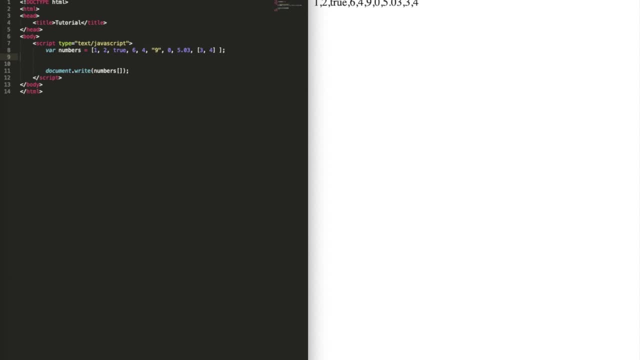 yeah, so in programming, uh um, it's kind of different. it's like the first element it would be zero. second element would be uh one, third element would be uh two and um so on. okay, so if you do zero, it'll print out one, because that's the first element. if you do uh three, don't print. 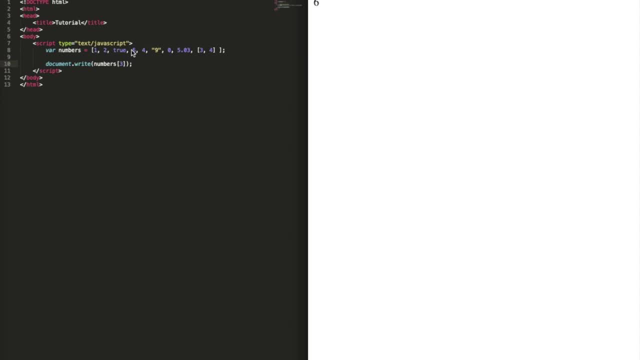 out the fourth element. so one, zero, one, two, three, okay, six, okay. so, uh, that's how it works. and um, yeah, so if you print out like um seven, you'll get 5.3, because zero, one, two, three, four, five, six, seven, five point, okay. and now, if you? 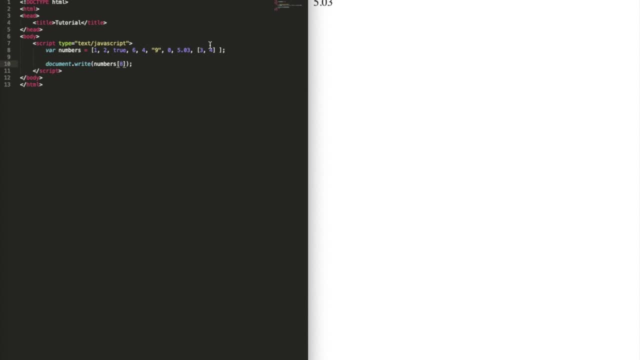 uh, want to do eight, which is the array inside the array. don't give the array which is three and four. but if you want to access um, an element in an array, which is often an array, then you can do two brackets and zero. okay, so that will do three and then, if you change that to one, 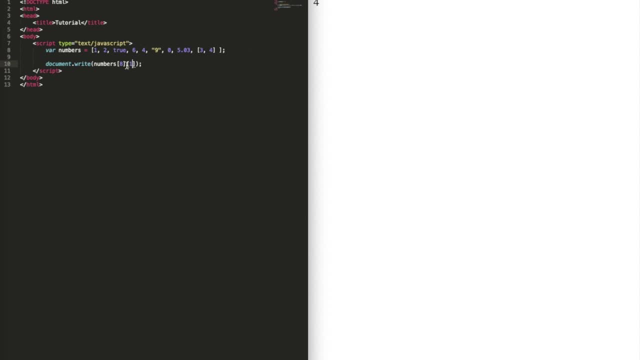 then that'll give four, okay, and uh, so on. and if you have like another um, if you have like a 10, but the array doesn't have a 10th element, then it's just going to get undefined. okay, yeah, so, um, yeah. and also, variable can also be equal to undefined, or it can also be equal to uh. 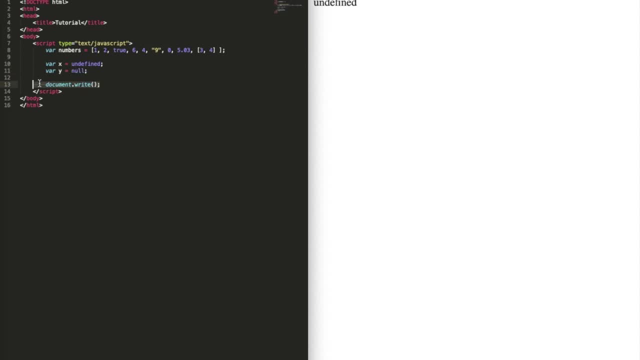 okay, they're almost the same thing and, um, it kind of makes sense: undefined. okay, because it's not defined, uh now. uh, since we did that, now let's go to object. okay, so var, my object equals to a curly brackets, and then click enter and then inside this object you have different properties. 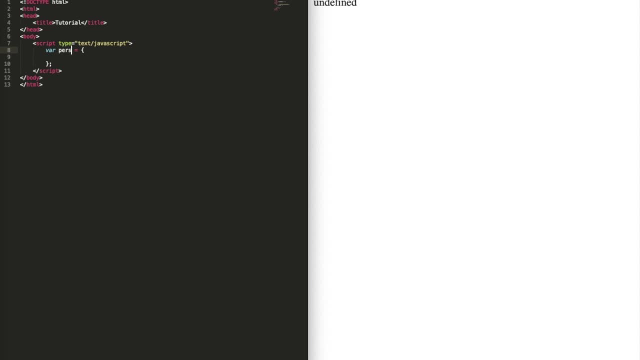 um, okay, versus do man? okay, first question. okay, so var person, because since it's also a variable, you can't do anything with var and uh, remember, you all have to end it with a semicolon. okay, now you can do name and then um instead of equals. you can do this thing and the name. 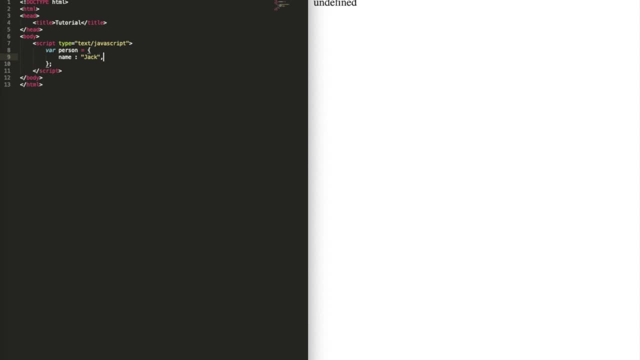 equals to jack. let's say the string, and then comma, age, um 14 comma, uh, let's say family or out of your parents, and then it's going to have an array: um, let's say bob and um sophia. okay, and then you don't have to put a comma here, okay, and then. so what you have to do, 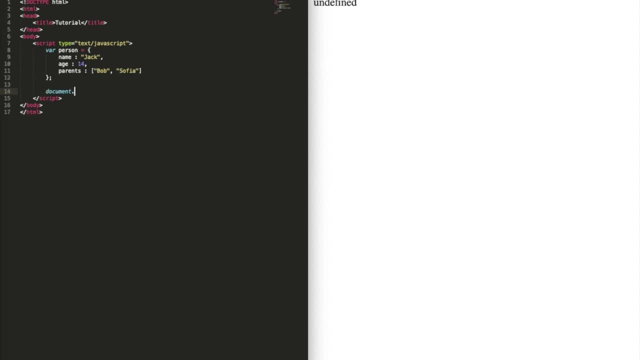 is you need to do uh to like get all the elements. you document it right. um, you can do person and then person dot name to access the name of it, and then jack and then person dot age- that'll get 14- and then person dot parents and then, since parents is an array you can uh access. 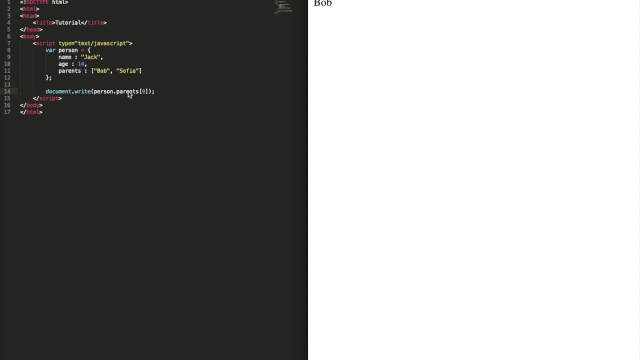 it by the square brackets. so if you do zero, then then it'll get bob, if you do one, it'll get sophia, okay, and then you can also make a sentence out of it. so you can do um person dot name plus um is plus person dot age plus. 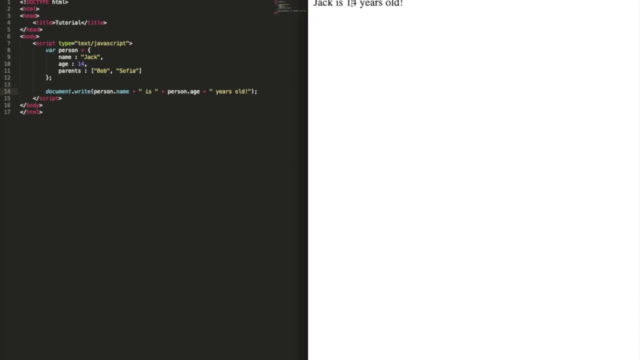 years old. okay, now i'll give jack is 14 years old, because the person dot name is jack, plus is plus person dot age, which is 14 plus years old. so jack is 14 years old. so, um, that was um the first part and i'll see you in the next part. so, yeah, see you, hey guys. so 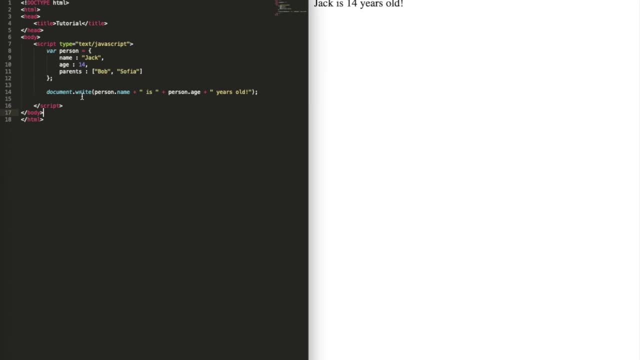 welcome back, uh, to part two. um, in part one, we learned like uh, things about the data types and arrays and things like that, and we also learned the documentwrite function. um, in part uh two, we're gonna be learning. um, we're gonna be learning about uh like other ways, like we'll be learning about. 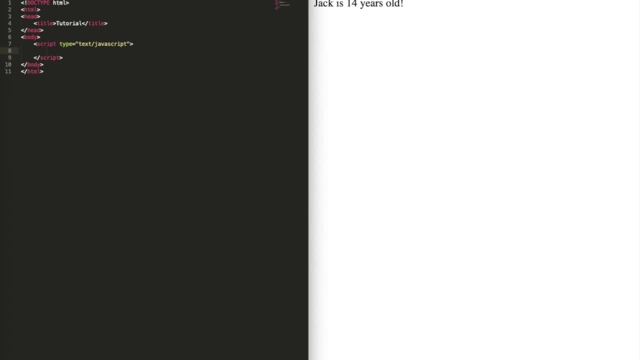 functions, object, object, instances and, uh, much more things. okay, so let's just get started. so i'm just gonna like refresh the page and the first thing that we'll look at it's called um something called functions. okay, so function is um, basically like a block of code. okay. 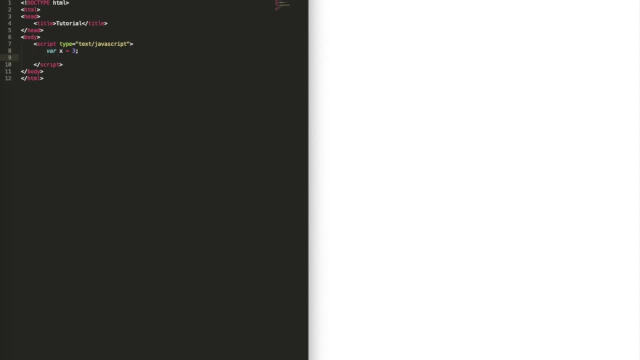 Like let's say you have a var x equals three and then documentwrite. okay, So like, that will give three. but instead of doing all of that, you can, yeah, yeah, so like, instead of, if you like, wanted to keep printing out like that. 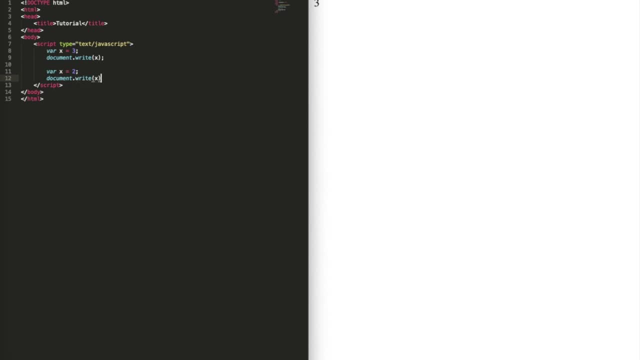 documentwrite rx. okay, Like if you want to keep doing that. it's kind of useless, but it's really inefficient. So what you can do is you can use a function. A function is basically just a block of code, okay. 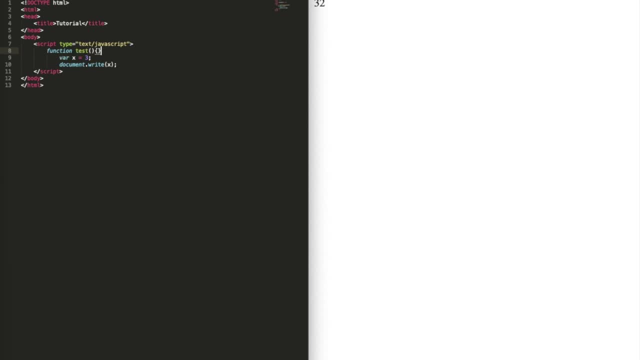 So function, test, and then you basically this is how you write a function- So the function and then the name of the function- mine is called test- and then two parentheses- I'll tell you guys what that is for later- and then a curly bracket and then all of your code inside. 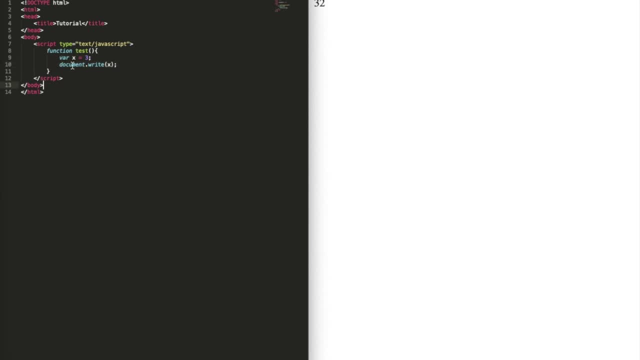 and then like exit, it's a curly bracket, So and then, if we run that, nothing will happen. okay, But that's because there's a block of code that needs to be run. okay, It's like we need to execute the function. okay. 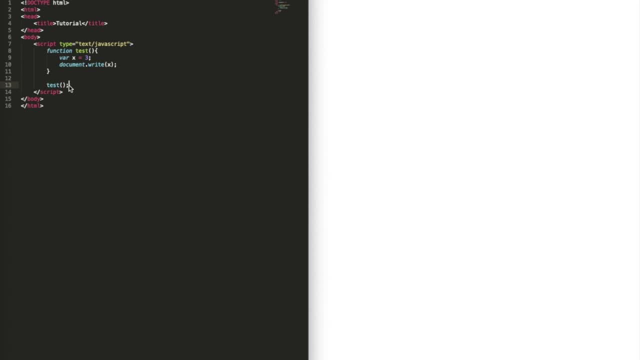 So you can do test and then two parentheses and then a semicolon, So that's how you like. run this block of code. okay, So that'll give three. And now, instead of doing var x equals three, like what, if we want to keep changing the value of x? okay, 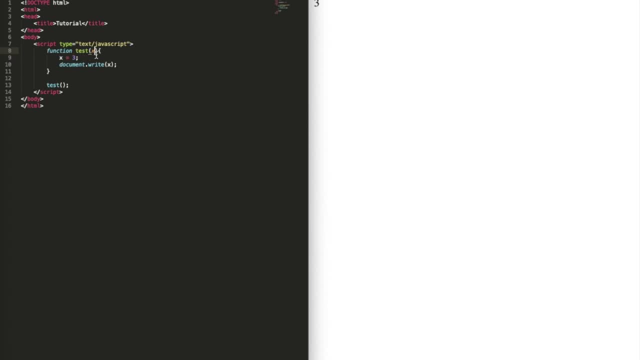 So like, instead of doing that, you can actually just put the variable name in the parentheses, okay, and then you can, over here, you can say, yes, you don't need this part. And then you can say: over here, equals five, okay. 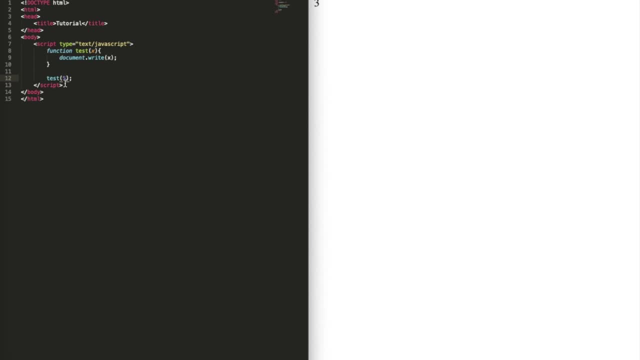 So now, yeah, so like this in this bracket it's basically saying that x is gonna be equal to five, and then you have to print out x. okay, Now that's five. And then if you do something like hello, I'll print hello, okay. 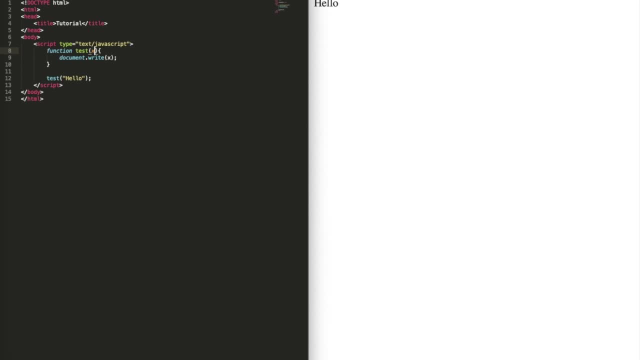 And then you can also have multiple. you know other other is how you run it, by the way. like these things inside: um global x, it's called an argument, okay. so like x, y, z, okay, and you can do um documentright, y and then documentright. 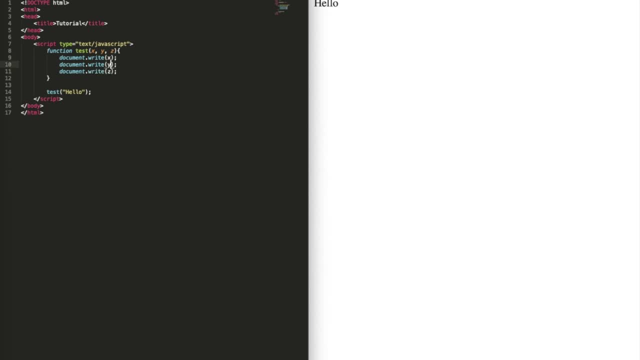 right, okay. and then obviously you can just have like a plus break and then plus break, plus break, okay. so, um, now you can uh go like this, okay. so like, when you do this, it says undefined. well, that's because we only give the value for hello, which is x, okay, for uh, x, which is hello okay. 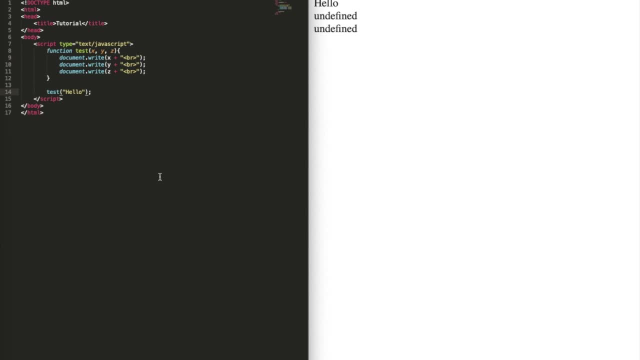 so. so it only printed out: um, hello. but now if you want to give multiple uh arguments, you can do a comma. i'll give it over here and then uh. so that was x, and now you're giving y. so y is one, let's say, and then z is, let's say, it's gonna be true. 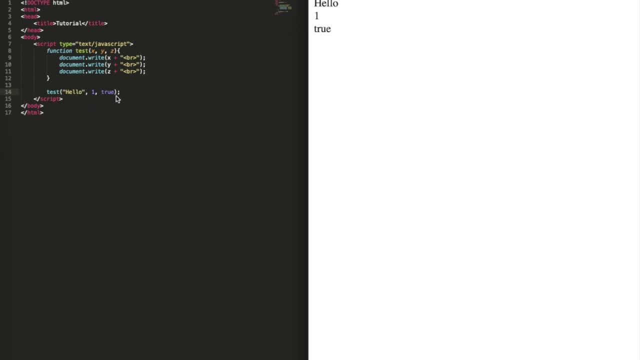 okay. and then hello one and true, so this is called function. okay, it's called function. um, syntax, yeah, and now um, you can also do something called return function, where you basically uh, just uh, return, oh, yeah, so like you can create a variable, let's say so var, um, let me just like. 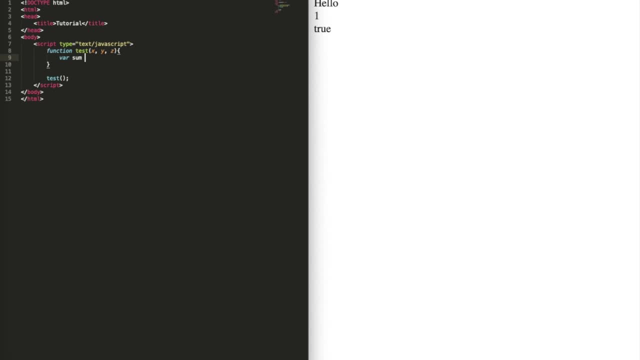 remove this. okay, so you can create a variable. let's say, for sum equals to x plus y plus z. okay, um, um, and then you can return some. okay, basically what this does, uh, the return function is just like um. whenever you call the function, the function will be equal to whatever, uh, this function. 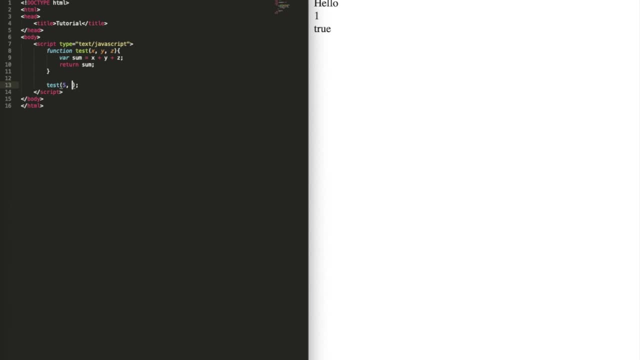 returns. so, for example, if you do test um five, four, three and nothing will happen, well, that's gonna be a document to write in. document is right, and then i'll give 12.. why? because first of all we put two arguments and- uh sorry, three arguments in the test. so what is five, four? 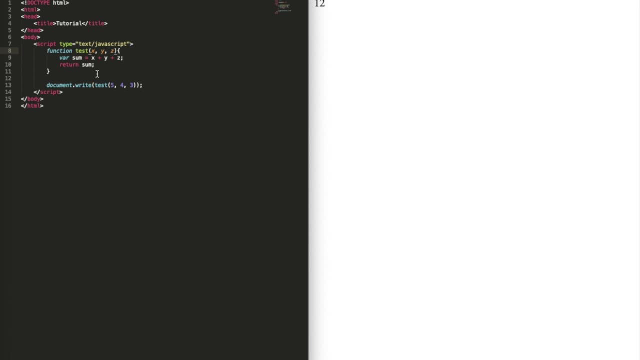 three, five plus four plus three is twelve. okay, so we calculated that using the sum, and then it uh said that well, this function is going to be equal to um 12.. okay, so like test five, four, uh, three is going to be equal to 12.. so document or write 12.. okay, 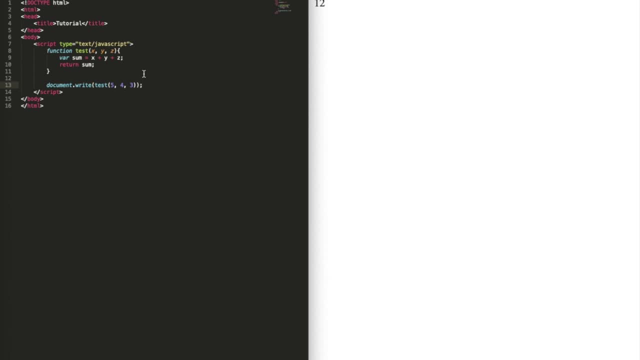 so, um, that'll function notation and then i'll move on to objects. so, guys, welcome back to part three of um. this video, and this video in part three is just going to show if statements and for loops and volumes. okay, so let's just go to if statement, for example, let's do. let's say: var x equals five. 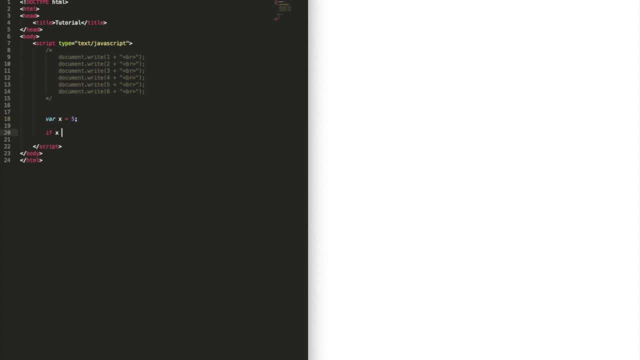 okay, uh, you can do. if x is um smaller than 10, then print sorry, then, oh my gosh, okay, okay, never mind if x, if x is smaller than 10, then document dot, right, uh, 10.. okay, and then document the right x. okay, then that's gonna print out five why. 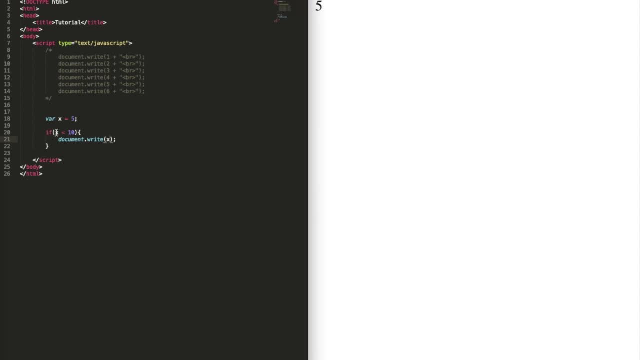 okay, um, because it's saying: if the value of x is smaller than 10- which it is because x is five and five is smaller than ten- then document dot right, x, okay. and if that's not true, so else, um, document dot right, um x. yeah, then, uh, document right, no, okay. so, um, if you have, let's say, 11, then i'll say no. 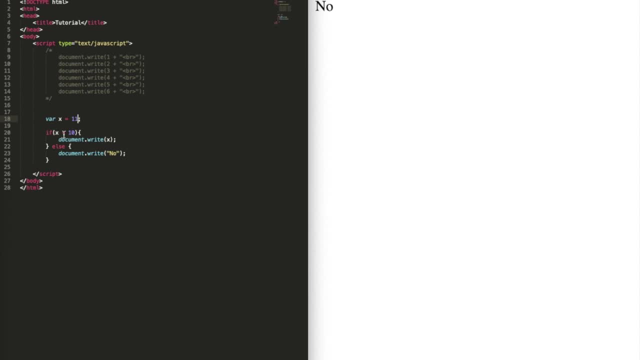 why? because, um, first it checks if, uh, 11 is smaller than 10, which it is not, 11 is bigger than 10, so it's going to go to else documentary right now. okay, so, um, there's also something called else if. so you can have else if. 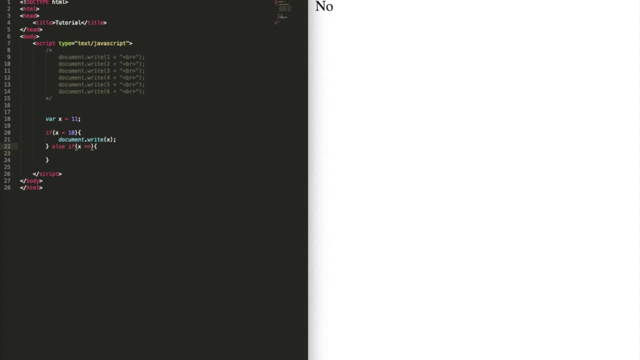 uh, you could do else. if um xd is equal to 15, okay, this how you check if something is equal to 15 or like equal to it. so like, if this number is equal to this value or this value is equal to this value, then you want to do a document. dot write 15 and you can do. 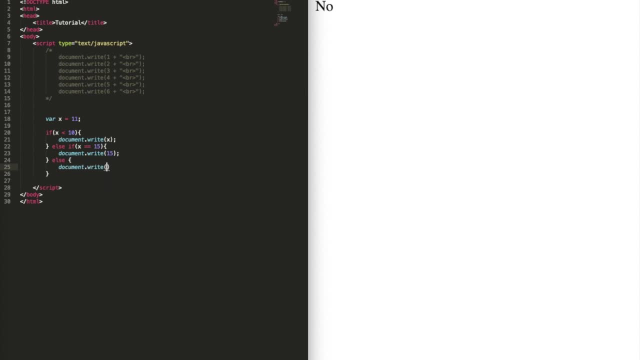 else document dot write 10 or no, okay, no, yeah. so basically how this works is: you have variable called X, first it checks and let's say, X is 1, okay, so if X is smaller than 10, which it is, then it prints out X, okay, so in this case it. 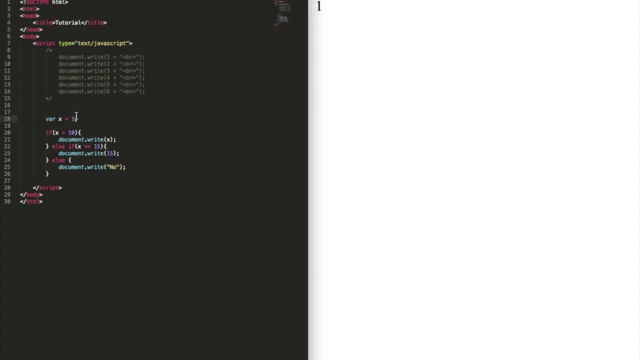 will print out 1, okay. but if X is equal to 15, then it's gonna print out 15, okay. so in this case, it will print out 15, okay. but if X is equal to 15, then it's going print out 15. then it's gonna print out 15. 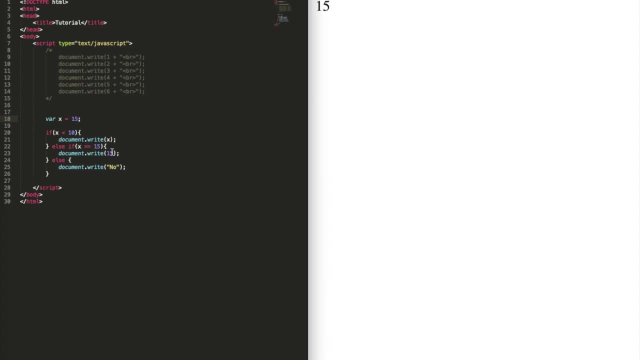 because else, if x is equal to 15, then do this. So x is equal to 15.. 15 is not smaller than 10, so it goes to this one, And 15 is equal to 15, so it prints out 15.. 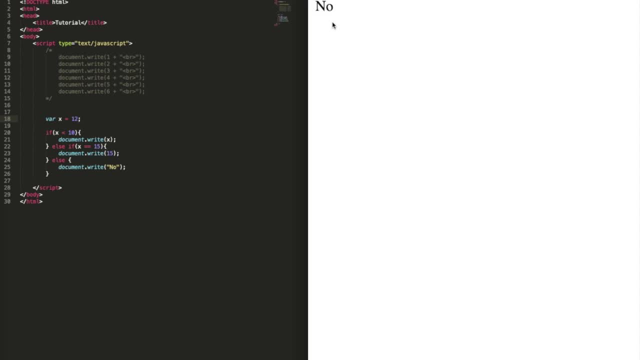 But now, if x is equal to 12,, then it's going to give out no. Why? Because 12 is not smaller than 10.. It's not equal to 15,, so else do this. So if none of these conditions are true, then do this. 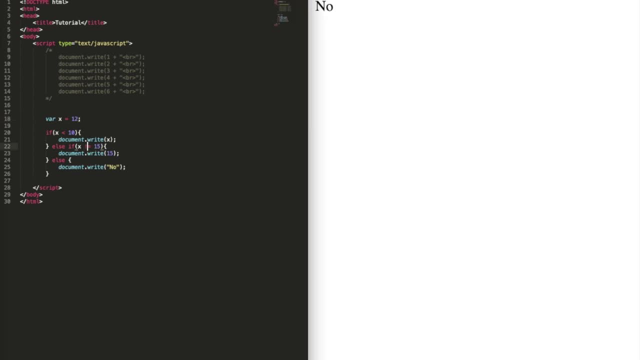 And you can also check: if x is not equal to 15.. So not equal to 15, then it will print out 15.. So this exclamation mark means not equal to. So exclamation mark and then equals, that means if it's not equal to. 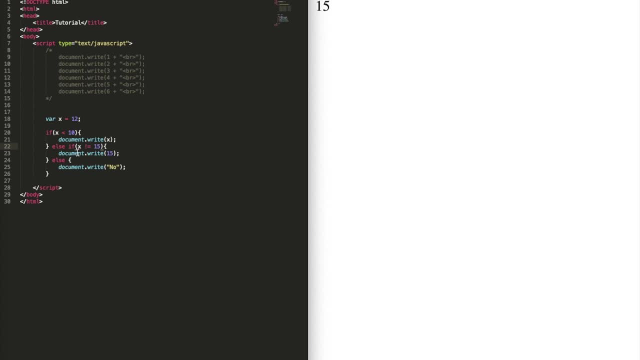 So 12, is it smaller than 10? No, so it goes here. Is 12 not equal to 15? That's true. So it prints out document or write 15.. Okay, And just skip this part. 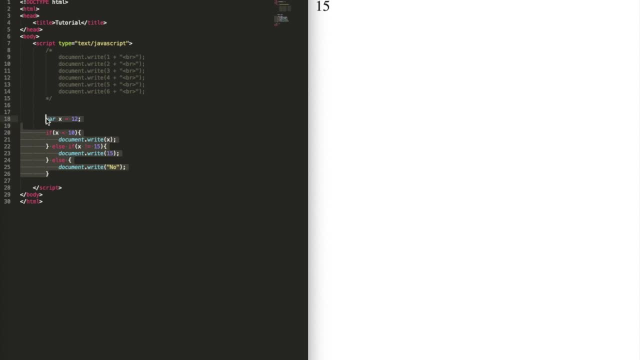 Okay, so that was if and else statements and stuff. So now what we're going to do is we're going to do switch statement. Yeah, so switch is kind of like else, sorry, if-else statements. So var x equals 3.. 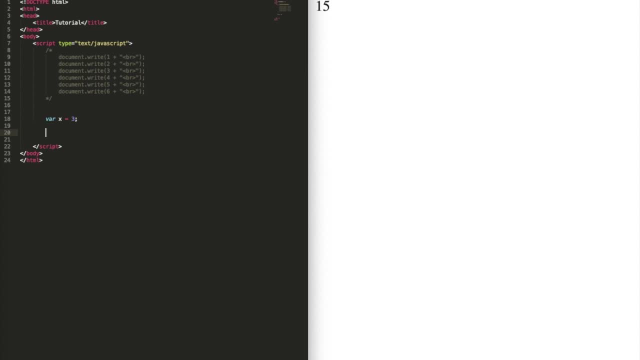 So instead of using, like many if, sorry, else-if statements, you can just write switch, Okay, so switch. So which variable do you want to compare? X? okay, And you can do case Case 1, documentwrite 1.. 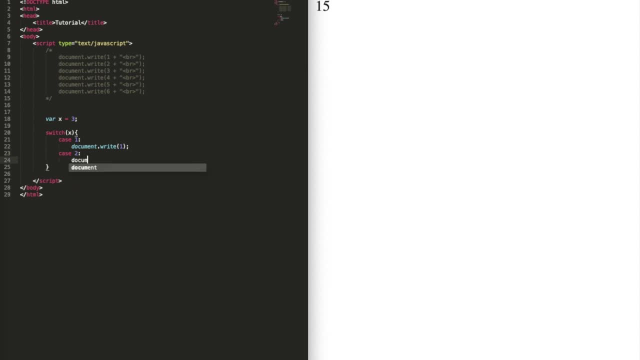 And then if it's case 2, then documentwrite 2.. And if it's case 3, then documentwrite, And then if it's case 3, then documentwrite 3.. Okay, And then you also need a break here. 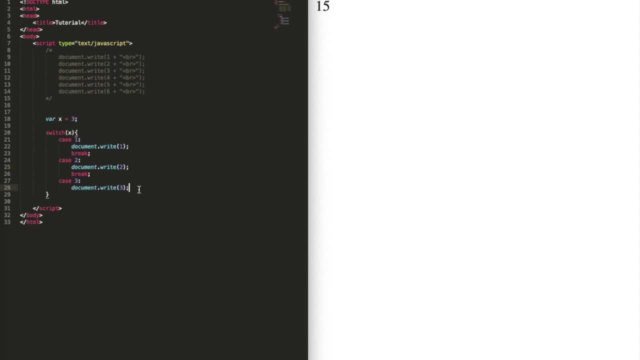 Break. I'll explain this a little bit. Right now just a second, And then default documentwrite other number. Okay, So basically what this says is that it compares x, which is equal to 3.. So if x is equal to 1, then print out 1.. 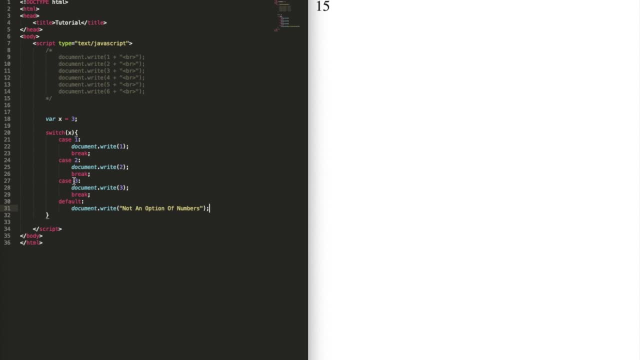 If x is equal to 2,, then print out 2.. If x is equal to 3, then print out 3.. And you also need a break at the end, okay, So let's see what this does: It prints out 3 because x is equal to 3.. 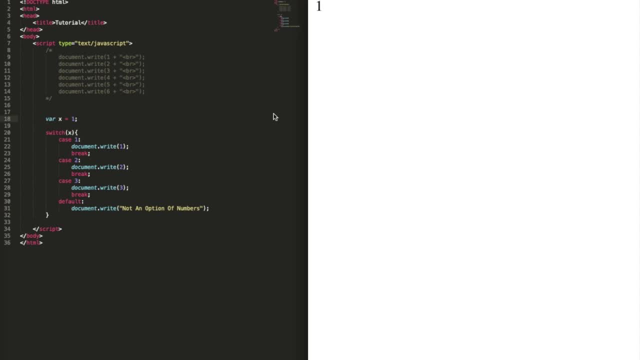 If we do 2, it's going to say 2.. And if we say 1, it's going to say 1.. Okay, But if it's If it's 5, it's going to say not an option of numbers, because this default is kind of like an else in the if-else statement. 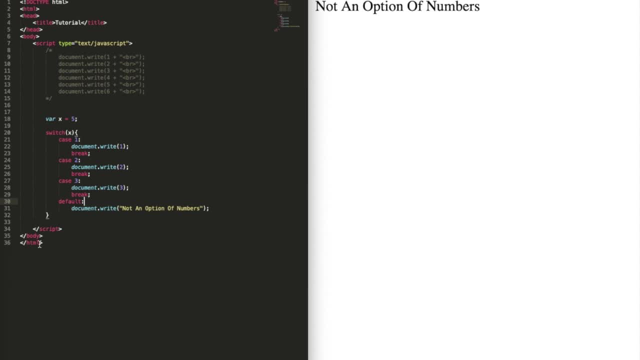 If none of the conditions are true, then run this: Okay, So that's switch statement. So that's pretty simple. And now what we're going to do is we're going to cover loops. Loops are really important, Okay. 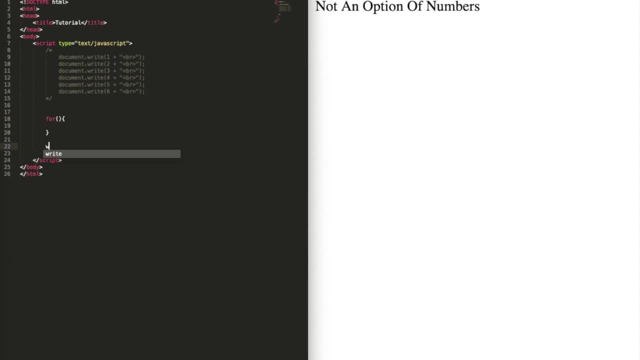 So for loop And this is also called a while loop. Okay, First I'm just going to look at for loops, because they're the most, They're the most commonly used. So basically the for loop and the while loop. they basically repeat something. 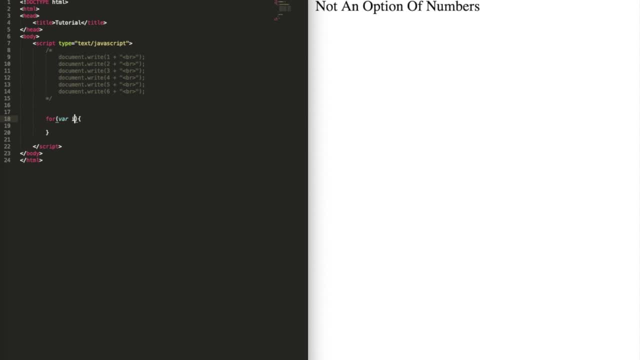 So this is how it works. So var i equals 0. i should be smaller than 10. i plus go documentwrite, i plus break. Okay, how does this work? So it prints out all this, But how does it work? 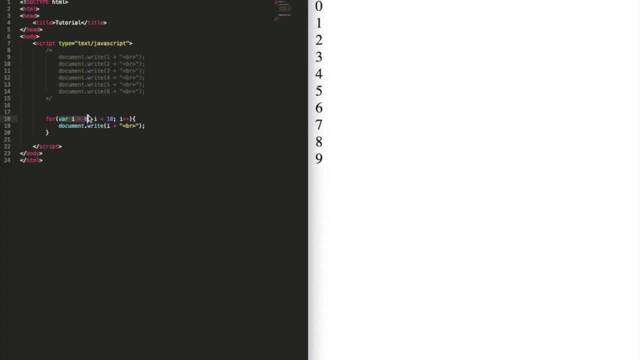 Okay, So it starts with a variable called i, Which is equal to 0. Then it says that keep increasing i by 1.. Okay, So plus plus is the same thing as i equals i plus 1.. And i minus minus is the same thing as i equals i minus 1.. 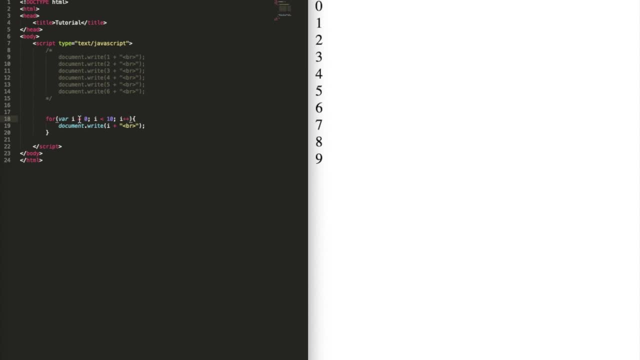 Okay, So we're just going to do i plus plus, So keep increasing i's value by 1. And then do this. Okay, So first it does var i equals 0. And then it does documentwrite. 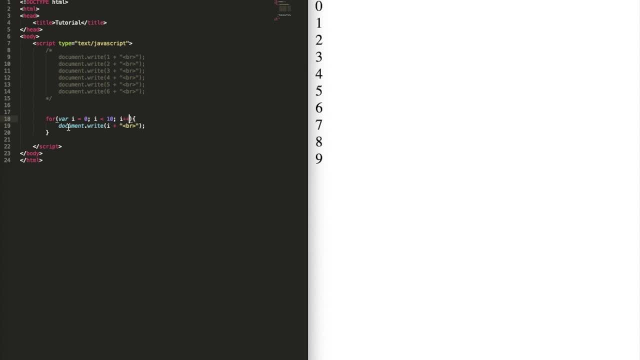 i, And then it increases i, And then it does this, And so on. It just keeps increasing i And then doing this, Increasing i, And then documentwrite, And then it keeps doing that until i is equal to 10.. 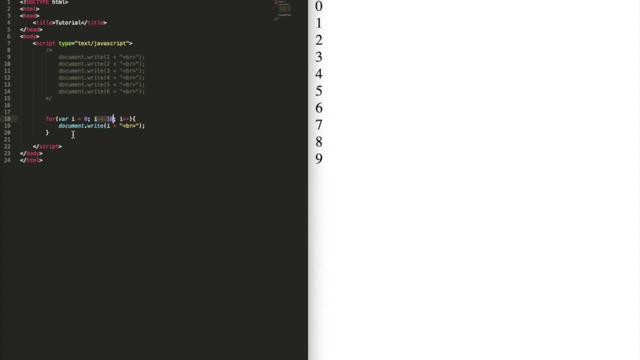 Because when i is equal to 10, the whole loop just stops. Okay. So that's how the for loop works, Okay, And then there's also a while loop, While loop, Okay. Okay, It's basically the same thing. 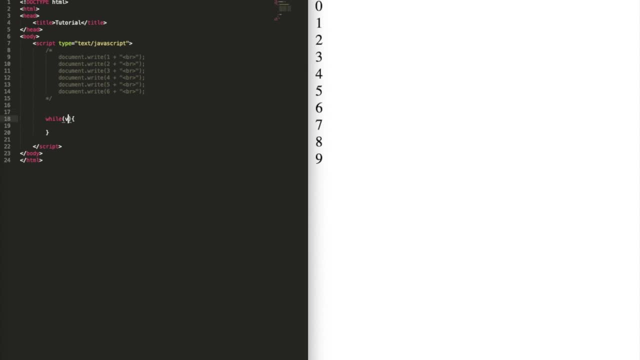 Kind of It. just, instead of putting a lot of things here, it has, it's kind of like, more organized. I guess I actually don't know, But var i equals 0. And it basically repeats everything inside it until this statement is false. 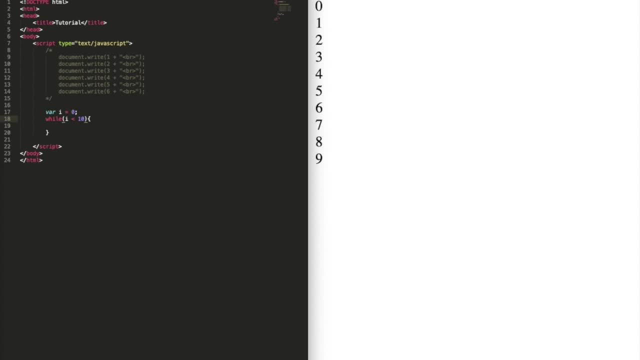 So i should be smaller than 10. And then documentwrite i plus break. Okay, Let's say i equals 1. And then i should be smaller than 11. So it can print all the numbers from 1 to 10.. 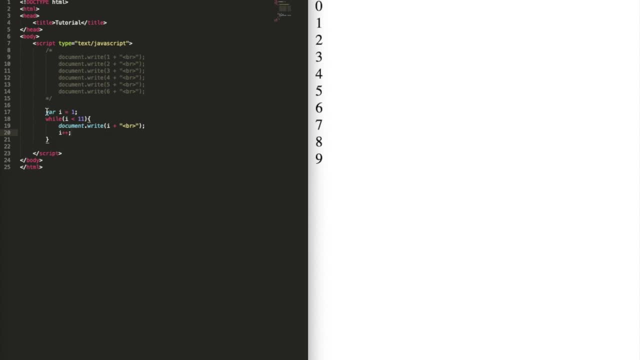 Okay, And then you can do i plus plus. So basically what this does: it starts by saying that var i is going to be equal to 1. And then it basically just repeats it, So it prints out i And then it increases i. 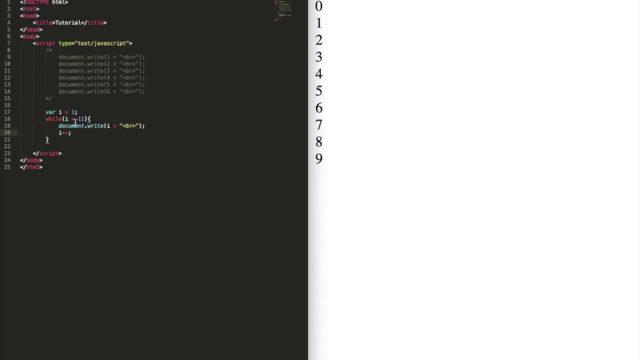 It prints out i, It increases i Until i is equal to 11,, where it just stops, Okay. Okay, So you can see that 1,, 2,, 3,, 4,, 5,, 6,, 7,, 8,, 9,, 10.. 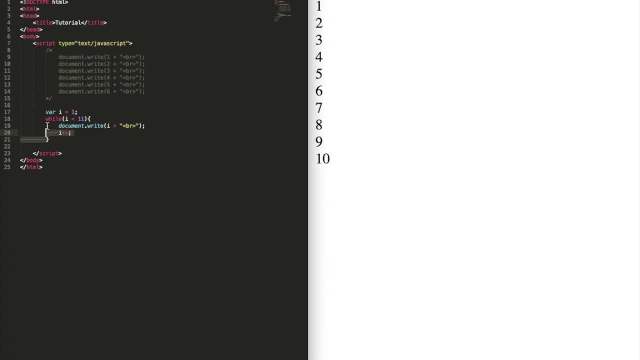 And then, when it goes to 11, it just stops. Okay, Now there are two keywords in the for loop and the while loop, which are called break and continue. They're pretty simple both of them, So I'm just going to go ahead and do 4.. 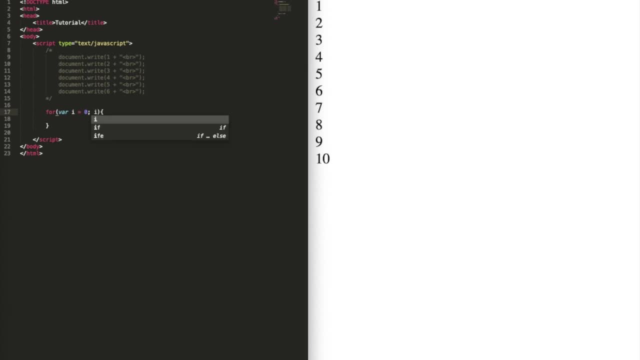 Var i equals 0. i should be smaller than 10. And i plus plus. Now we can do So. this basically just prints all the numbers From 0 to 9. So plus vr, And then 0 to 9.. 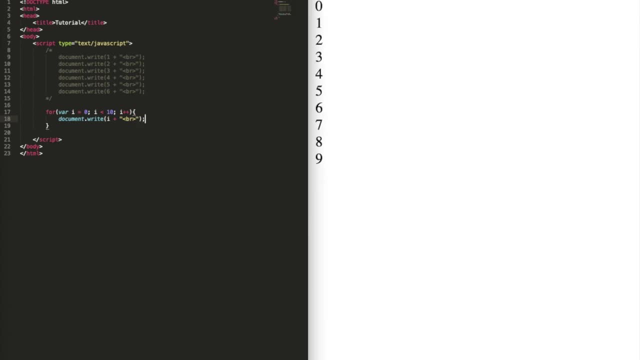 Okay, But now what we're going to do is we're going to use the break and continue, Okay. So if I'm actually going to put this up here, Because we just learned the if-else statement, So I'm going to use that- 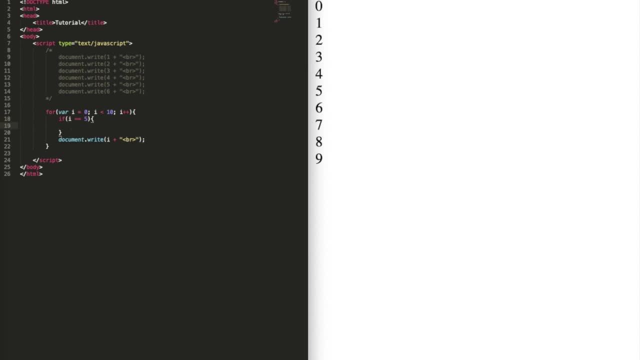 So if i is equal to 5. Because we want to skip 5. Okay, Then continue, Continue, And then You can see that 5 is not there, Basically what the continue thing does. So the program. 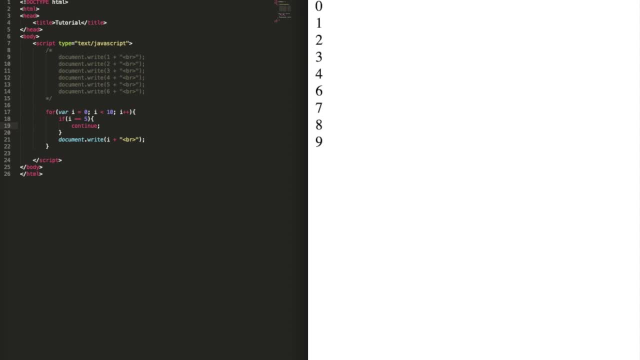 It goes from up to down, by the way, Like the computer reads it from up to down, Like we do, And Yeah, So it Like it keeps printing out i, And then it comes across this For every single element. 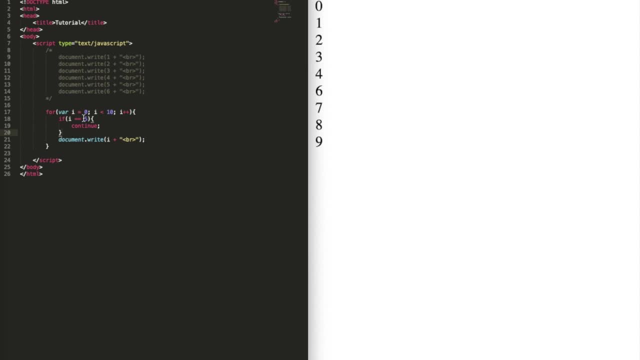 So, for example, if i is equal to 1.. Is 1 equal to 5? No, So it just does this, Okay. But if i equals to 5., Then continue. What continue does It basically just goes back at the top. 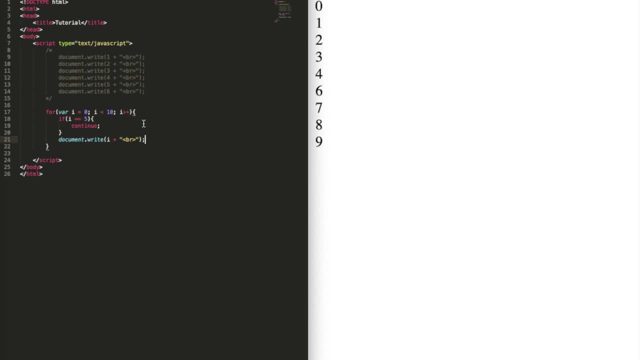 And it increments i And then just prints this. It kind of just skips the element, basically Okay, And then break. Break just stops the whole loop. Okay, So if you do break, Then at 5. It just breaks the whole loop. 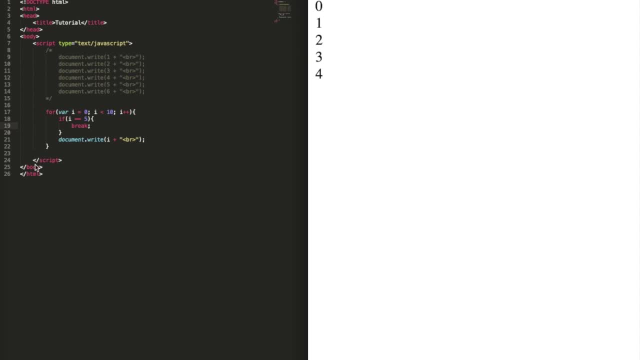 Okay, So you can't see anything. So it just like stops the loop. So those are for loops and while loops. Oh, and one more thing: You can also use Array operations with loops. For example, if you have an array called bar numbers equals to 5,, 3,, 2,, 0. 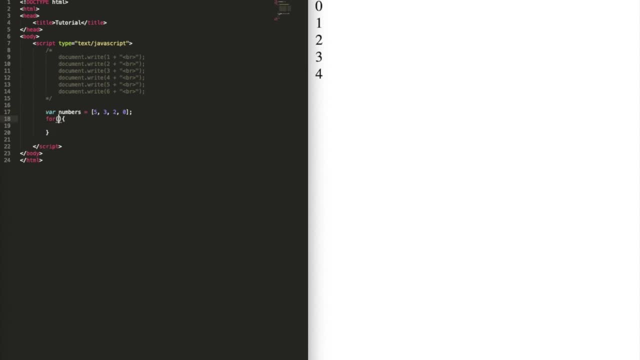 And then you can have a for loop that basically iterates through all the numbers. So bar i equals 0.. i should be smaller than numberslength. That's like a new keyword. So the length thing, It basically just returns. 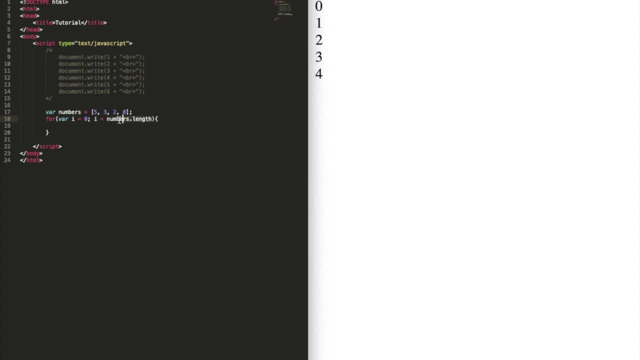 Or like this thing over here: Just set to the number of elements that this array has. So numberslength, That would just be 4.. Because numbers has 4 elements. So you can see 5 is 1.. 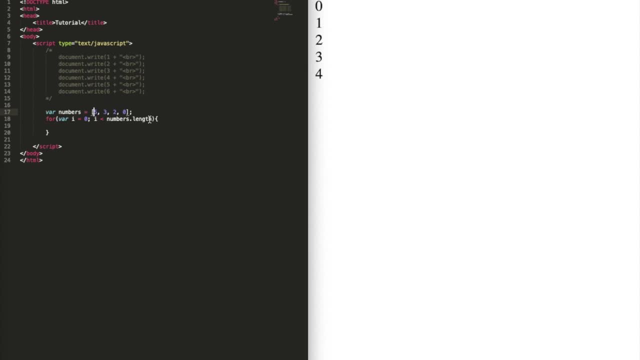 And then 3. And then 2. And then 0. So that's 4 elements. Okay, So numberslength is equal to 4. And then i equals plus. Then you can do documentwrite. 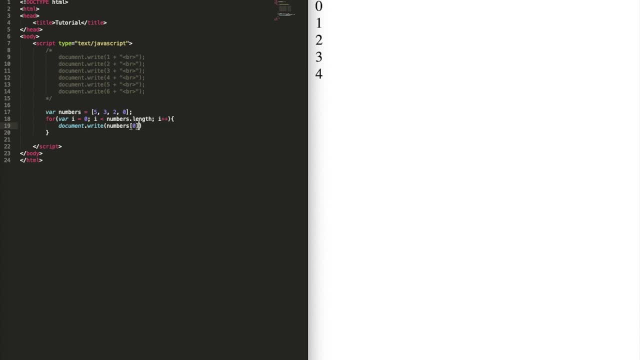 Numbers And then insert viewing 0. Because then That will just do. I'll show you: Okay, That will just do: 5,, 5,, 5,, 5. Because numbers of the 0 is always 5.. 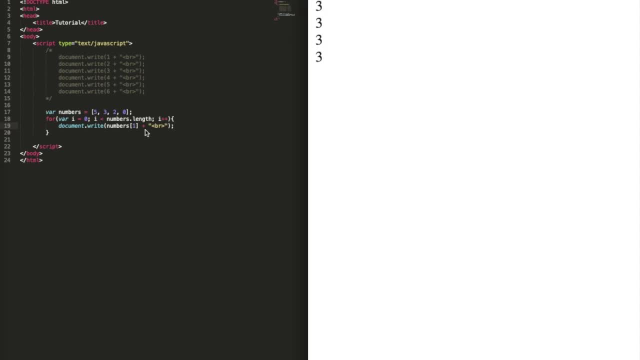 Okay, So if you do numbers of the 1., That will be 3., And if you do numbers of 2., That will be 2.. And then if you do numbers of 3., That will give 0.. 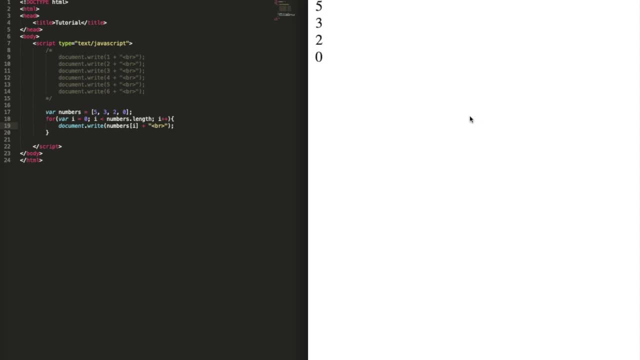 Okay, But what we want to do Is we want to do i, And that's just going to print out the whole list. Okay, Because it starts with 0. And then it prints out numbers 0 to 5.. 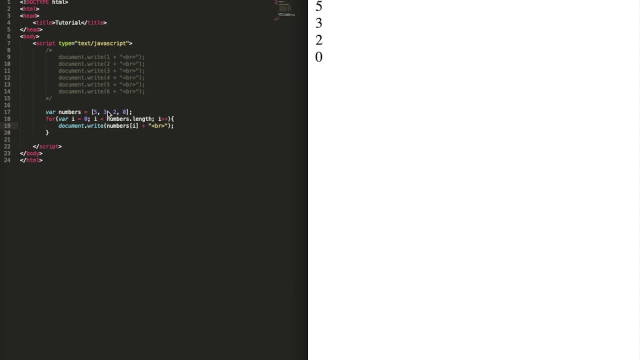 And then it goes to 1.. Okay, And then it prints out number 1,, which is 3.. And then it goes to 2.. And then it prints out number 2,, which is 2.. And then it goes to 3.. 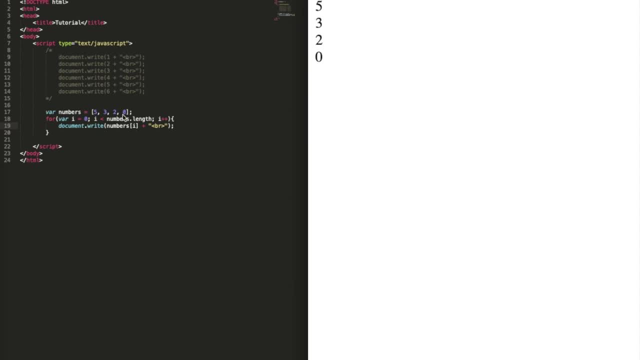 And then it prints out numbers 3,, which is 0.. Okay, So that's array operations with for loops, And now we are going to learn how to connect HTML with JavaScript. Okay, So yeah, Let's just go ahead and do that, I guess. 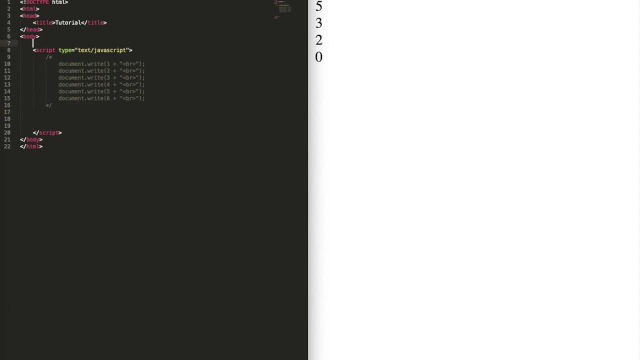 Yeah, So, like I said, you need to know HTML for this. Let's say you have an input, So input type equals text, And then the ID is going to be Bob. So yeah, So to ask, like, as you can see over here, 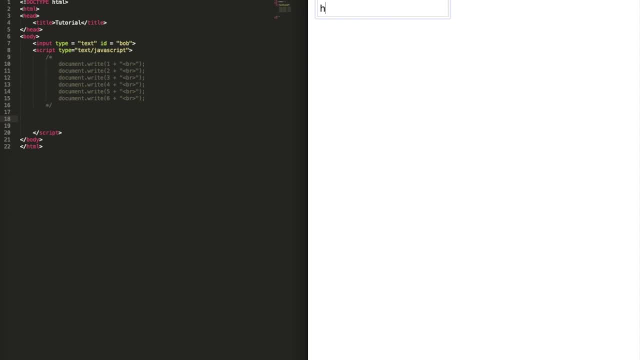 What we just did Is we made an input field So we can type anything here, So like to like, yeah, And then let's say we get a button. Okay, So button, click me Okay. 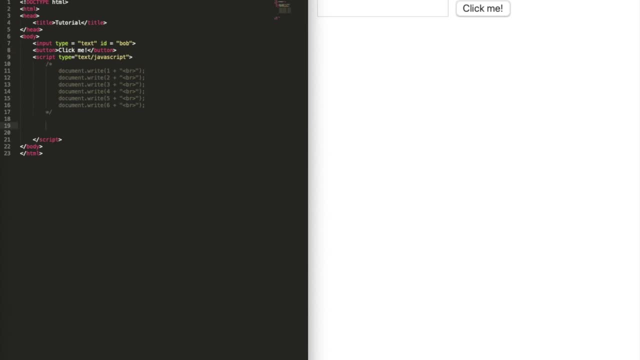 And then there's a button called click me. Okay, So what's going to happen is we're going to do onClick, So like, when this button gets clicked, you basically run a function Because, like we learn functions called, you can name it anything. 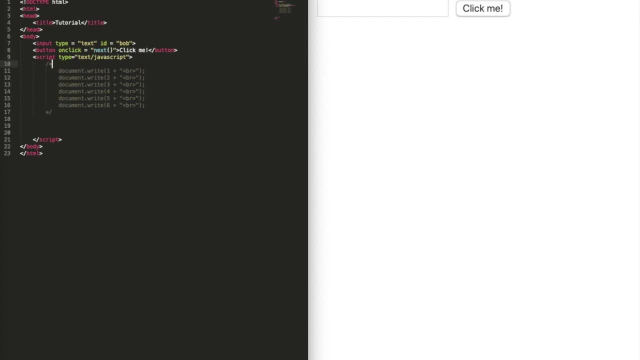 Let's just say next, next, okay, because it does the next thing, all right. and then, oh, we actually have to define the function, so we need to write up the function. function next. what's gonna happen now? it's really cool, okay. so what we're gonna do is we're. 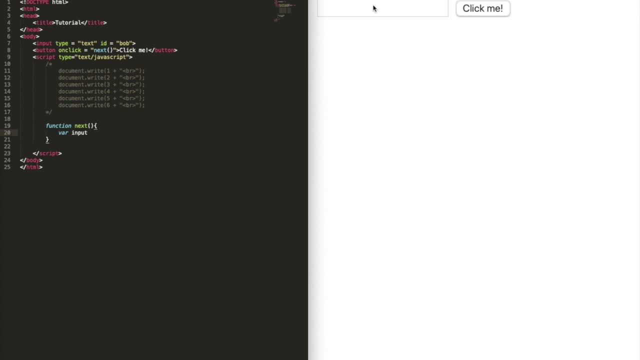 gonna do for input. so like we're gonna get whatever the user input, okay to do that. we import equals to document. dot: get element by its ID. okay, and what is this ID? its ID is Bob, so we're gonna do Bob, okay, and then dot value. so the value. 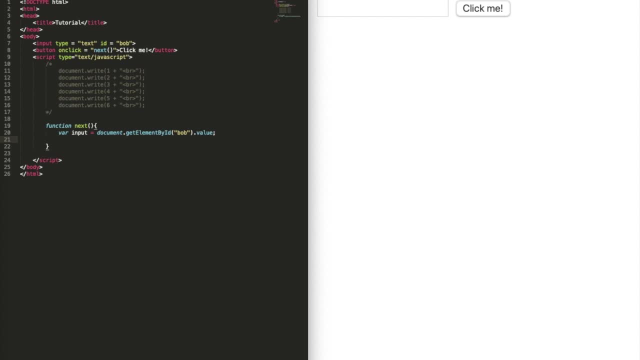 of: okay, so now we can do alert, because that's like another way of document alert input. okay, now let's say we type in hello world, check me and say hello, okay, basically what it did is whenever we click the button it runs. this function called next and this variable: it gets the document. 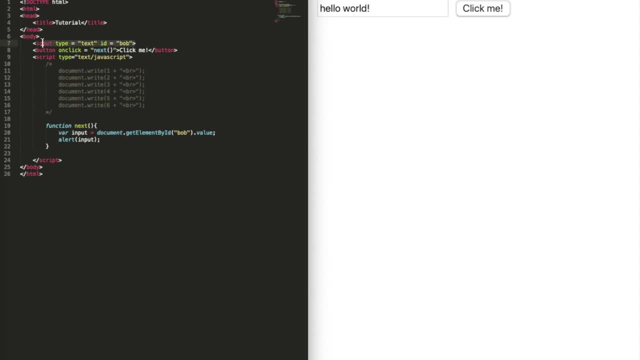 the input, like whatever the user input in from the input tag, and then it alerts it. okay, yeah, so that was how you get things from the HTML document. or you could also do query selector, so query select selector. but, um, now, right now it wouldn't work, so let's say hello. 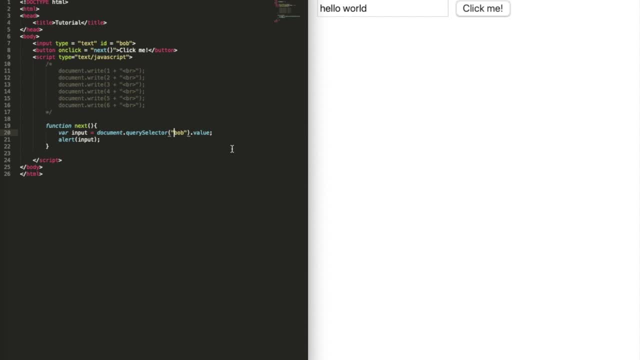 world. it wouldn't work, okay, cuz query selector. it's not like dot: get element by ID, so you don't specify the ID. okay, and HTML CSS and JavaScript: you specify ID by using a hashtag. okay, So now you can do the world and then that okay. 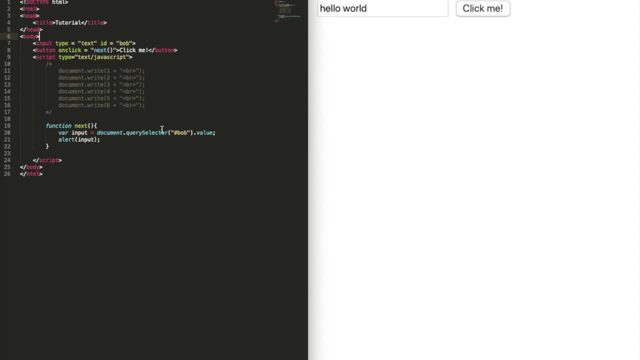 And now you can also do class name. So let's say this class is equal to Bob, So you can do document. Yeah, so documentgetElements. Remember that S, because you're getting several, because the class can get a lot of things. 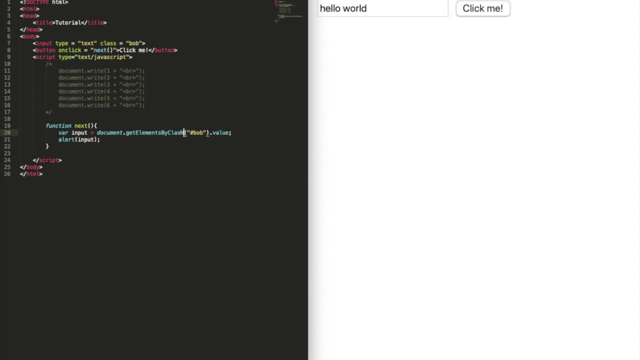 unlike an ID by class name: Class name And then the class name is Bob, But this also wouldn't work. Hello world, Undefined, okay, And this is why, Because, basically, let me see something. Yeah, so basically, since there can be lots of class elements, 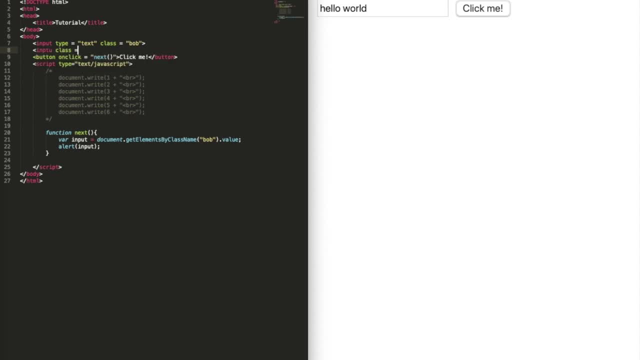 so let's say we have another input and then this class is Bob2,, okay, And then, since there are two elements with Bob, this basically gets an array. okay. So Bob0 is what we want. We have the first element in the array, okay. 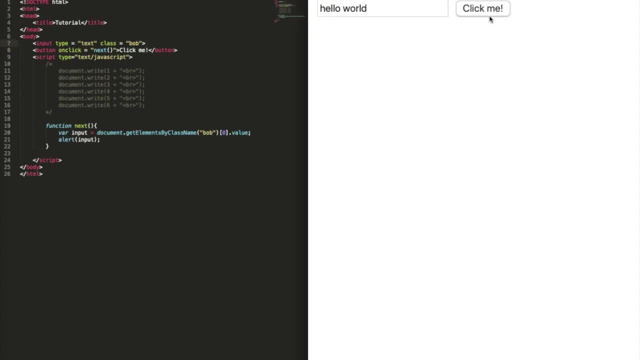 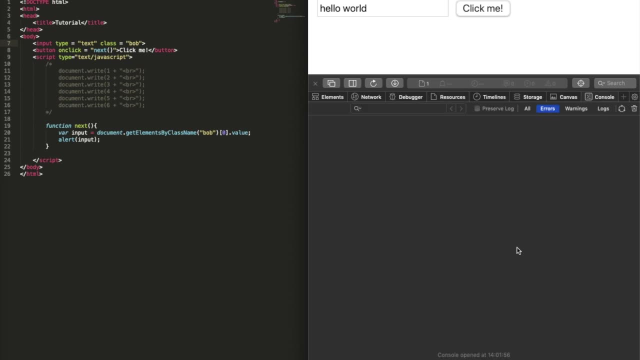 So Yeah, and then that will print out. hello world, I'll show you guys how it works. so Console, Yeah. so if you do documentgetElements by class name and then if we do, Bob, as you can see, it returns an array of inputs. 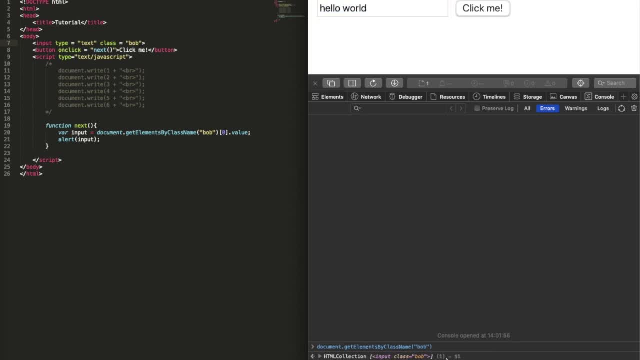 So with, Yeah, with one. like the array only has one element, which is this input. So if you want to do this thing, so var x equals to. So for a second, var x equals to that. okay, And now to x. 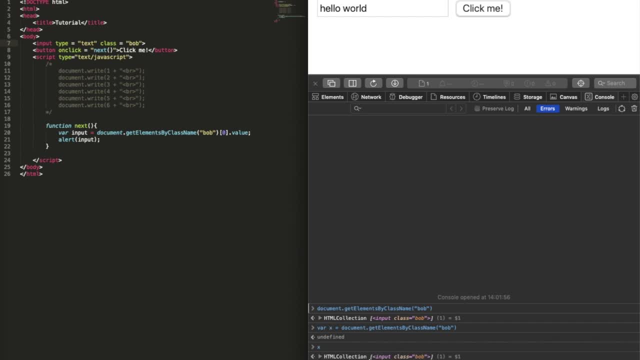 We will get the array of like elements with the class of Bob. So if we do x 0, then we get this element over here. Look, I'll do that again and you can see over here. Yeah, yeah, well, okay. 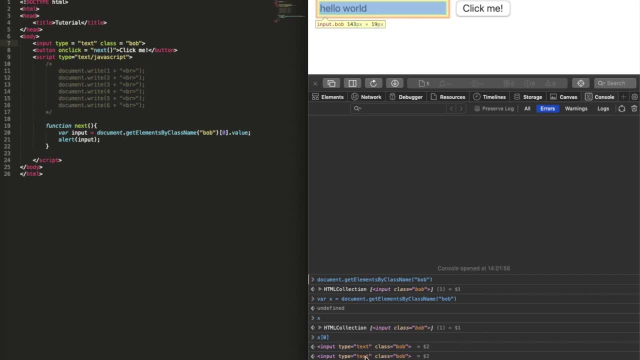 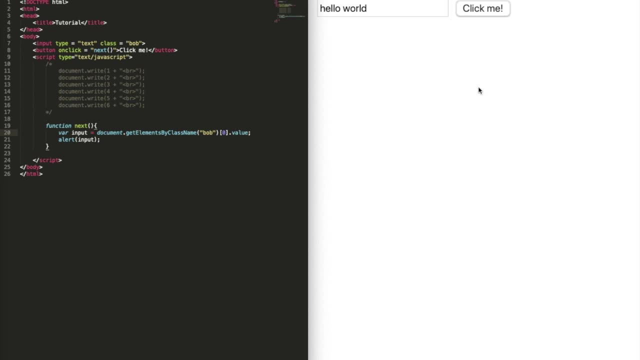 So basically, yeah, you can see over here it's pointing at the input box. okay, So that's how it works. So, which is why we need a 0, because it's an array, basically. So, Yeah, that's that. 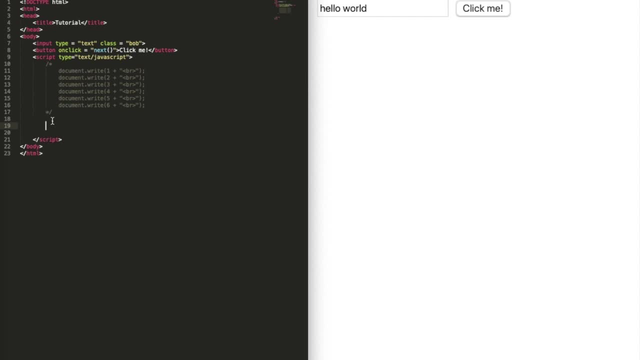 And then we also will need function objects. okay, That's going to be a little tricky, so you really need to pay attention, okay? So basically, like we learn objects like var object and then equals and name and so on, okay, 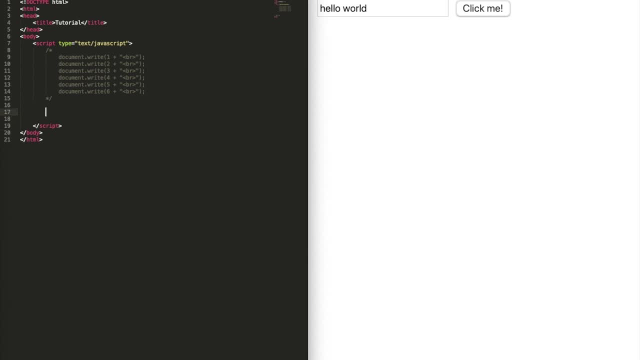 You can create an object like this. okay, Like there's another way of creating an object, So I'll say function, person. okay, This is called a Structure function. This is how you create another object. okay, Now you can give this person a name and an age. okay, 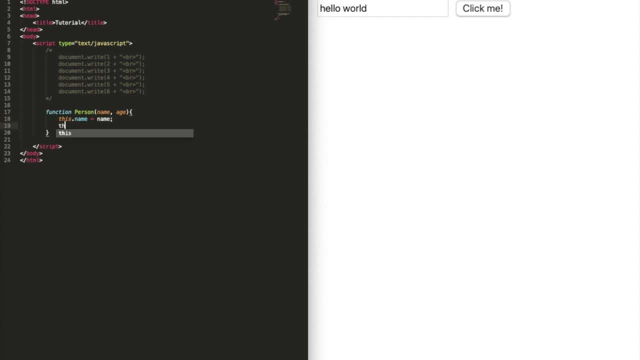 So this dot name equals name, This dot age equals age And that's how you like. make sure that the user, like you yourself, who's typing this code, will later give these values, okay, But if you want to make sure, or if you make sure that the values are constant, 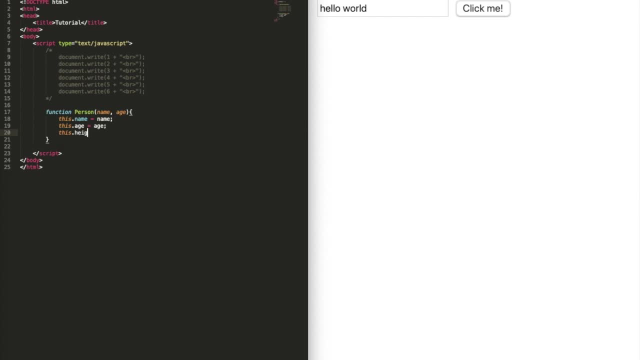 then you can do this dot. for example, height or weight equals 53 kgs. okay, So these are like the arguments of the function. okay, And this is like just a variable in the function. okay, And you can do this dot function. so this dot say equals to a function, okay. 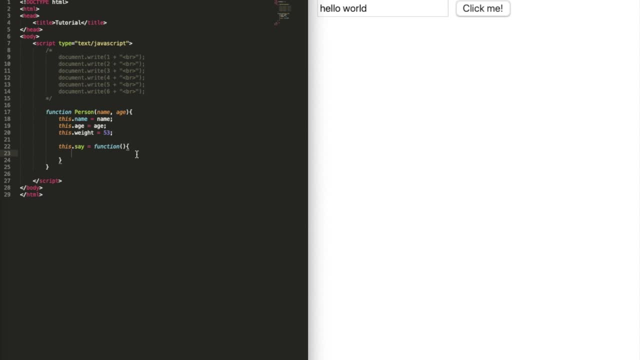 You can do that. So this dot say is a function, And then we can do document, dot write This dot name plus is plus this dot, age plus years old, And is plus This dot weight plus kg. okay, So now nothing will happen. 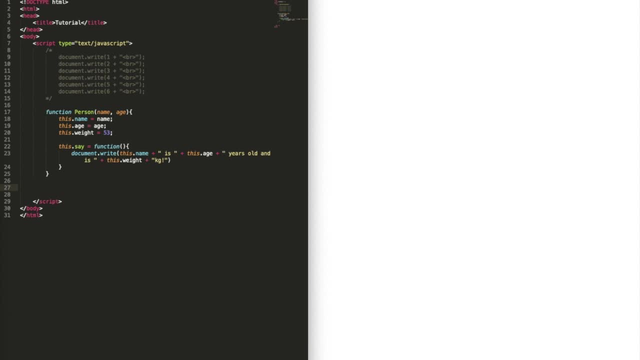 Well, that's because we need to create an object first, okay, So let's create different people. So you can do this by doing var. let's say person1 equals to a new person. okay, And his name- that's the first thing- is going to be, let's say, Jack. 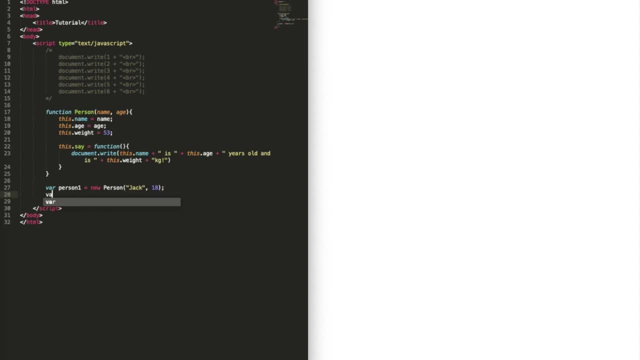 And his age is going to be, let's say, 18.. And var person2 equals to a new person, And let's say his name is Bob And his age is 29,. okay, Now we can actually do person1.. 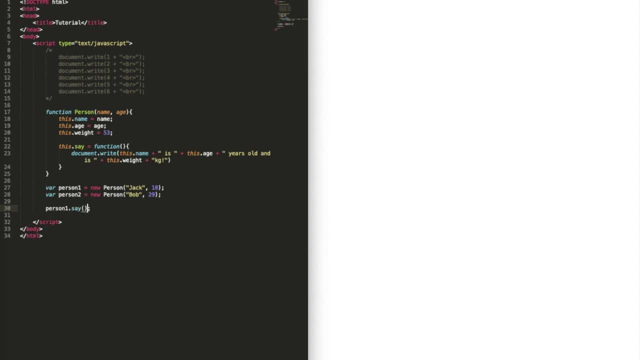 Yeah. so person1 dot say okay. So, like for person1, he has a function called say okay. Person dot say: And then Jack is 18.. And then Bob is 18 years old and 53 kgs. 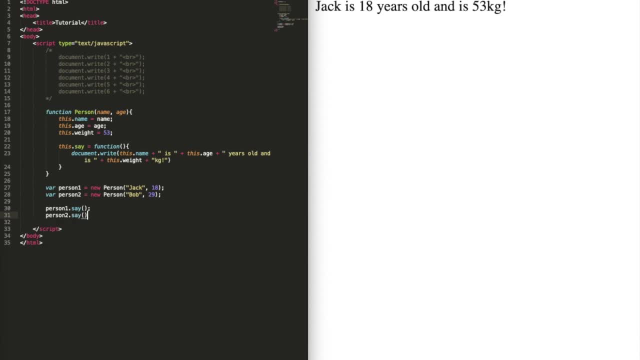 And then we can also do. person2 dot say, And then it says Bob is 29 years old and 53 kgs- okay, And then we can also change the values. So we can do, for example: yeah, So we can do. I'm also going to have a break over here. 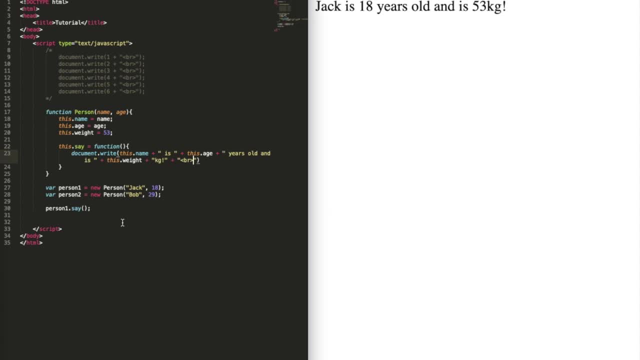 So plus break, okay. Okay, so I'm going to do Yeah, so you can also change the values, So you can do this dot weight. So, not sorry, not this dot weight, but person1 dot weight equals 60 kgs. okay, 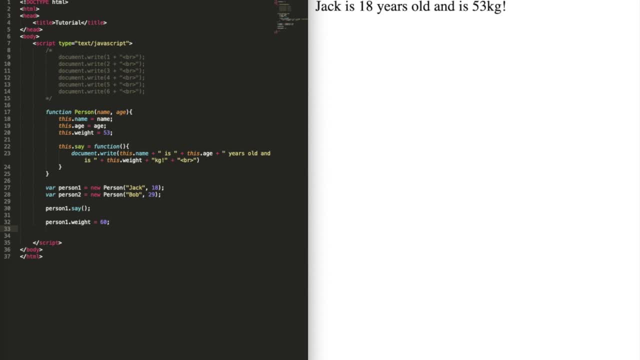 So he got another 7 kilograms. okay, Person 1 dot say So. now you can see how it changed. So Jack is 18 years old and 53 kgs, And then we change the value. Jack is 18 years old and 60 kgs. 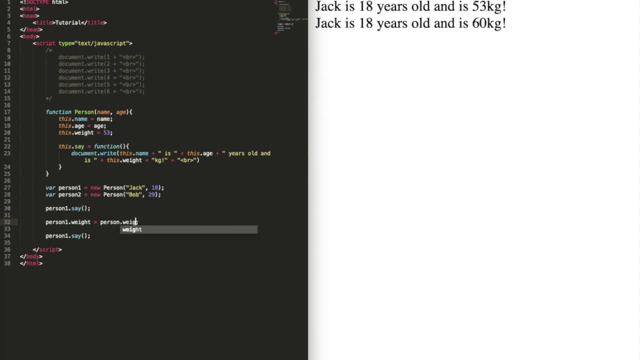 You can also do this by doing Like incrementing it, kind of So plus 7,, okay. So then that will: Oh, person1 dot weight, yeah, And then 60 kgs, And you can also do plus 10, along with 63 and so on. 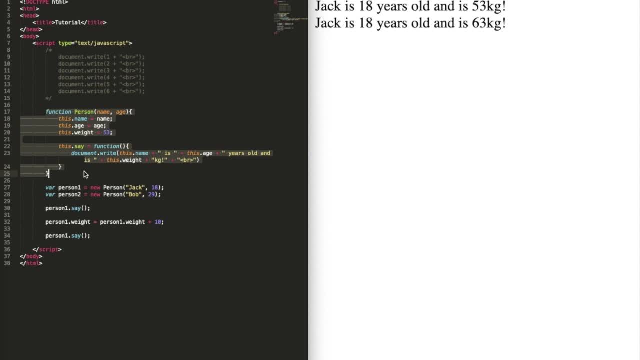 So that's how you create like a. This is called a function constructor or constructor function, And this is called an object instance. okay, So yeah, And then you can check if This object is an instance of this function. So you can just do that by doing document dot write. 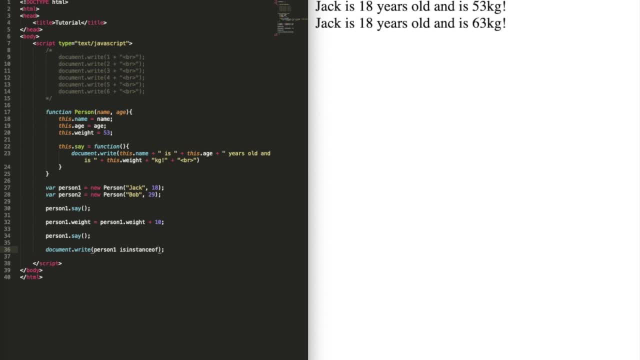 Person1 is instance of Sorry. person1 instance of person, okay, And I'll say true. But if you do, for example, person, Yeah, so person2 is also 2.. Sorry, true. And then let's say you have another variable. 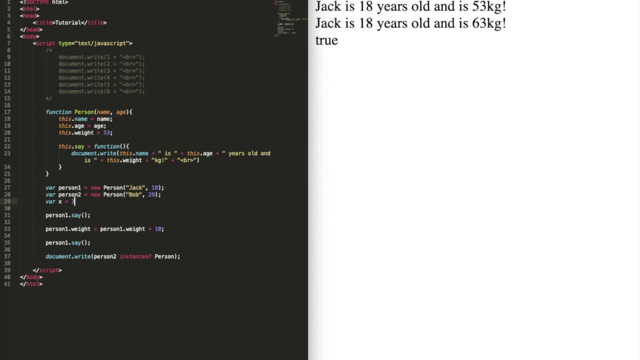 This is a variable called for. x equals 3.. If you do x, dot is false, False. okay, It basically checks if this object is made from this constructor function. okay, That's what it checks. So that's object. Yeah, whatever. 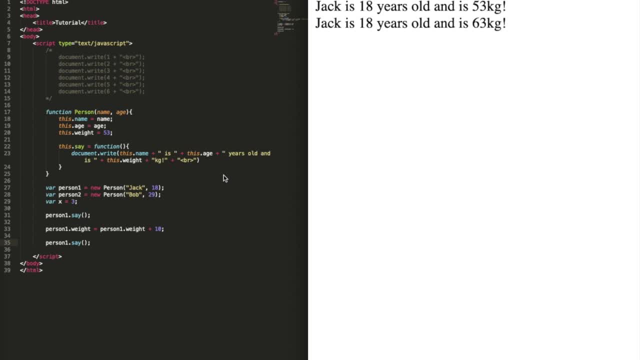 Okay, Constructor functions and stuff. What else did you cover? Um, Okay, Oh, yeah, Okay, So I'm just going to delete all of this Refresh. So we learned document dot, get element by id and things like that. Now what you can do is you can actually import other libraries and stuff. 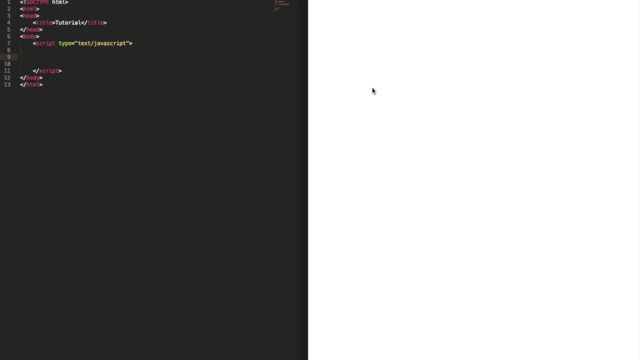 And a library is kind of like a module, basically that helps you do a thing, For example, if you make games. it helps you make games, It uses JavaScript syntax, But it basically just like teaches you how to. It doesn't teach you, sorry. 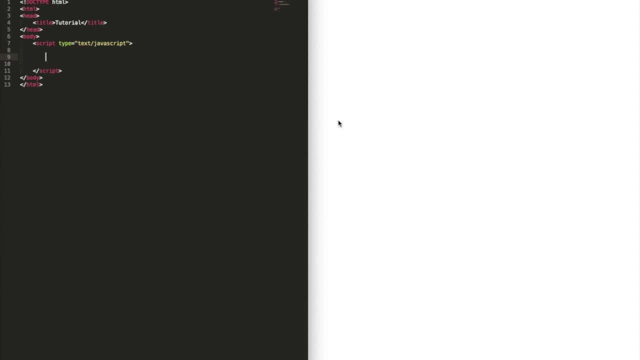 It helps you in making a game better. For example, let's say in JavaScript, if you want to create like a canvas- it's basically like where the game is happening- You need to write like a ton of code. 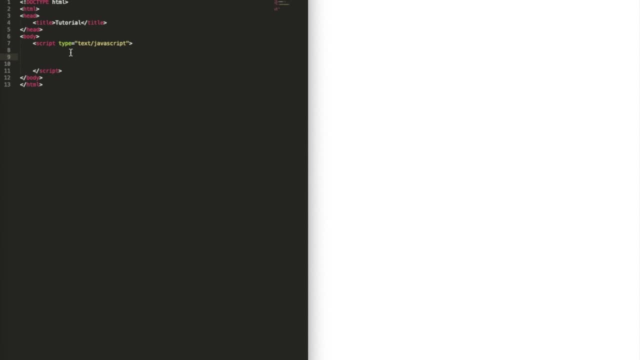 But if you import a module, then you can just like, Then you can just like: do it like in one line, okay. So that's, It's basically like easier, okay. So I won't be. 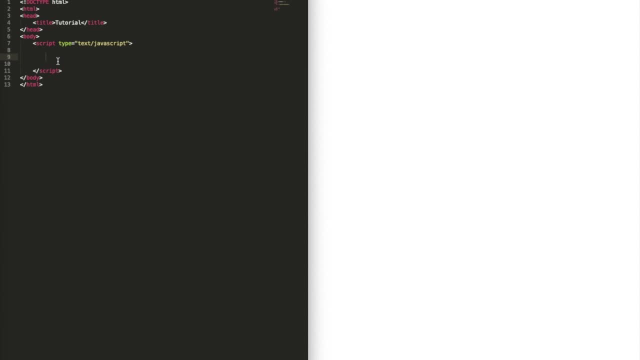 I won't be teaching them this tutorial, but maybe another one. okay, But I have another thing in mind. It's called JSON. okay, Now, JSON is really important Because it basically stands for: So that's JSON, It stands for JavaScript. 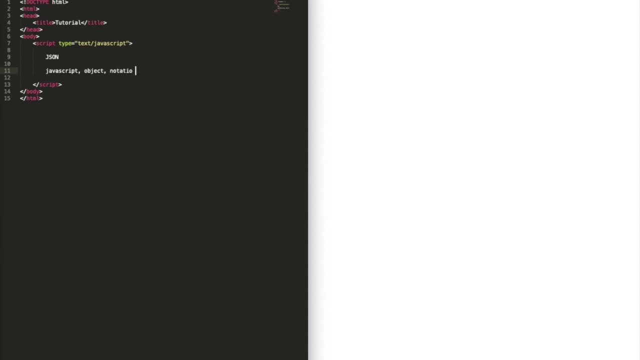 And then object And then notation. okay, And now I'm just going to show you guys how JSON works. Oh, Here we go. Okay, So JSON. it's basically like, Let's say, you have a new file, Call it testjson.